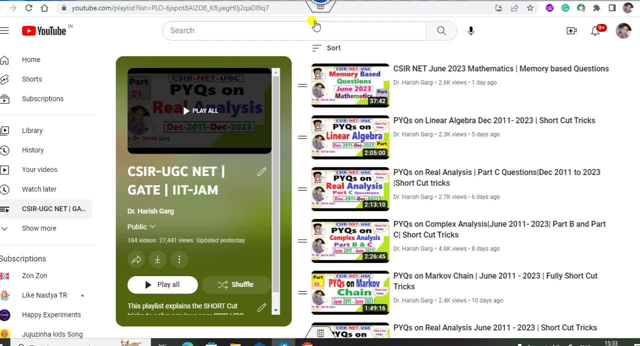 my WhatsApp group for the various discussion. What you will found on my YouTube channel? there is a playlist of the CSR UGC net. Here you can found the previous year questions. that is a memory based question. previous years, last 12 years papers- solution related to the 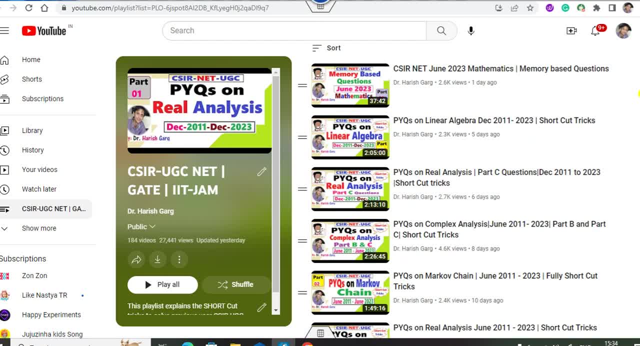 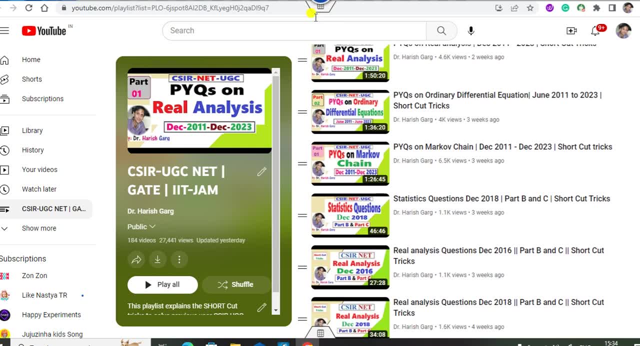 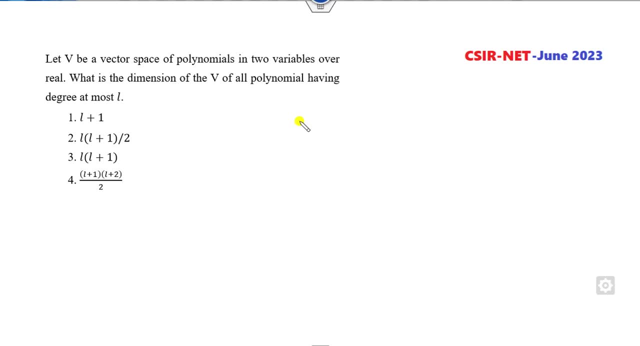 linear algebra, differential equation, real analysis, complex analysis, partial differential equation and many more. all are you can see in this playlist. So we can see now in this part we will see about the June 2023.. So the first question is related to here. 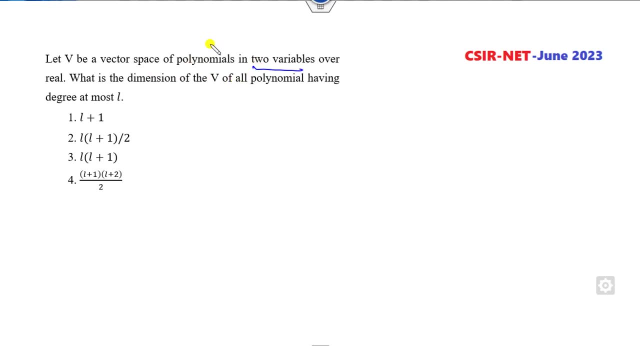 V is the vector space of the two variable. it is a polynomial of the two variable, like x, comma, y Over the real. then what is the dimension of at most l? That is a very simple how you can think about that. So, firstly, I can tell you a simple shortcut tricks based on which you can find any. 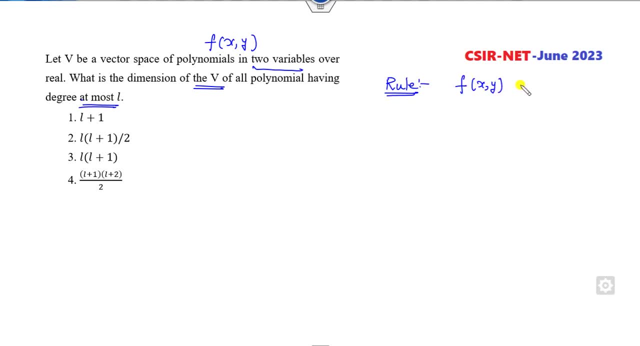 of the polynomial of degree here. So if I say this is my at most degree, n, then the dimension, the general formula, will be n minus number of the, n plus number of the variable, combination number of the variables. For example, if I say in this case, how many variables? Two variables, So this is my two. 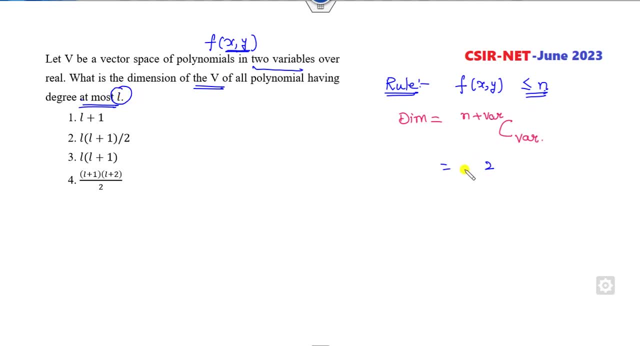 What is our degree? at most l, It is at most m, So it is a l C number of the variables. So this is the right answer. So if you open them, it is l plus 2, l plus 1 over 2 factorial. So 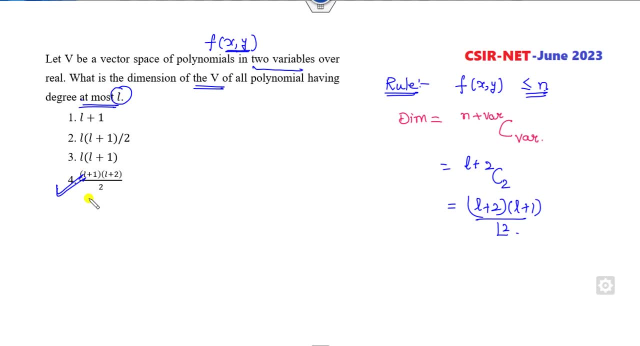 you can see which is there. This is the right answer. Otherwise, you all knows, a degree of polynomial x, comma y is at most the 2.. What are the bases? 1, x, y, x, square y, square, x, y. You can see how many variables are. What is. 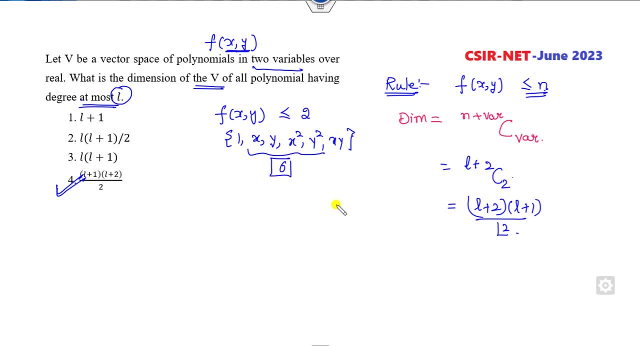 the degrees 6.. Dimension is 6. And if you apply this formula again, l is my 2.. So 2 plus 2 is here, So that is my 4c2, again 6.. If you want to find a polynomial of 3 variable, at most say my: 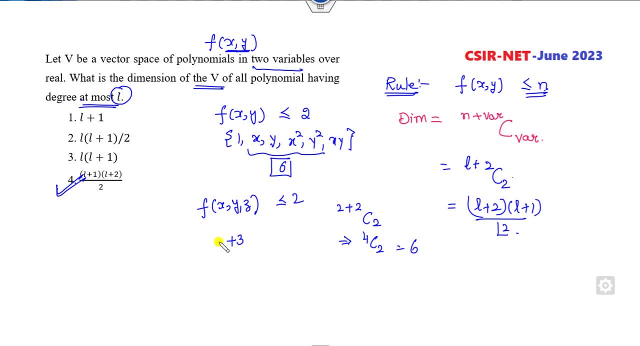 2.. Then number of the variables are my 3. Degree, at most 2. 2 is my here, So that is a 5c3.. Again, 5c3 is nothing but my 5, 4 over 2.. That is my 10.. So 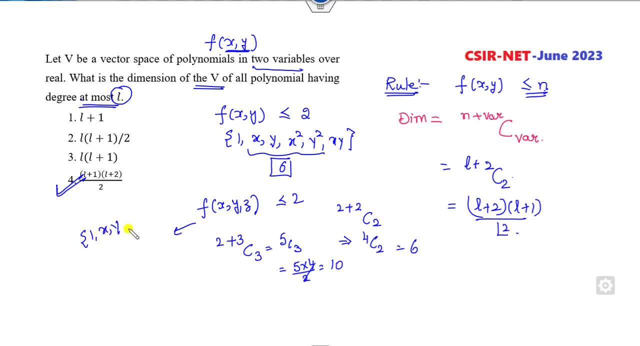 what are the bases? If you write like 1, x, y, x square y, y square xy, x square y, y square x and y cube, So how you can see 3 plus 3 plus r. here You can see this is the y is repeated. 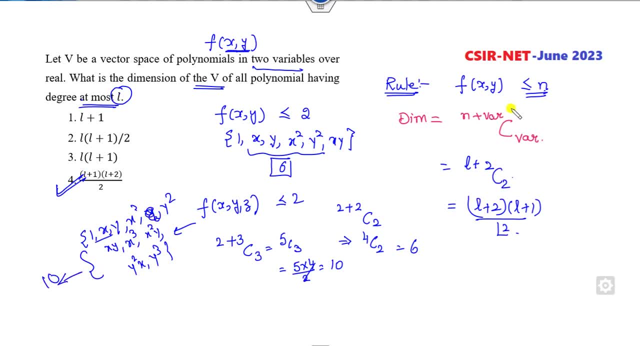 So there are the 10 pair r. So this is the simple formula. You must remember it whenever you have to find a polynomial degree less than equal to n. So accordingly, you can find this question here. So this is the general formula. You can solve it. You can also see if I say polynomial. 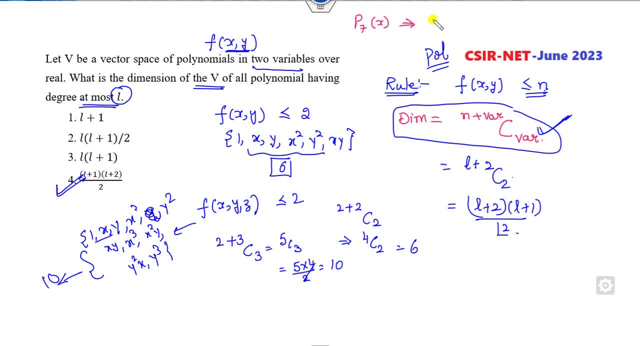 of degree 7 of the single variable. What is the dimension is 7 plus 1, 8. And if you look about here, n plus 1, c of 1. Again, it is n plus 1.. So this formula is applicable. It is a general. 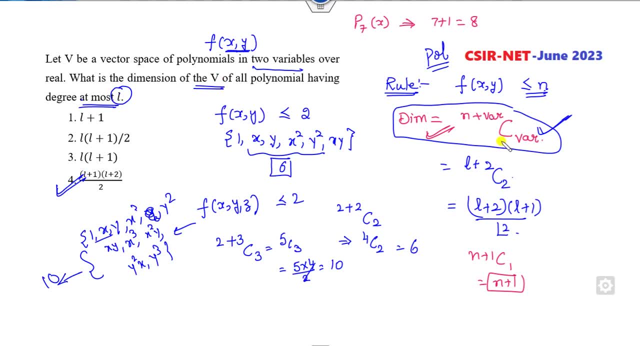 formula for finding a polynomial of degree less than equal to n. So this is the general formula. So this is the general formula for finding the dimension of the v. So I hope this formula will be helpful for you in this coming examination as well. Okay, look at this another one. A is a. 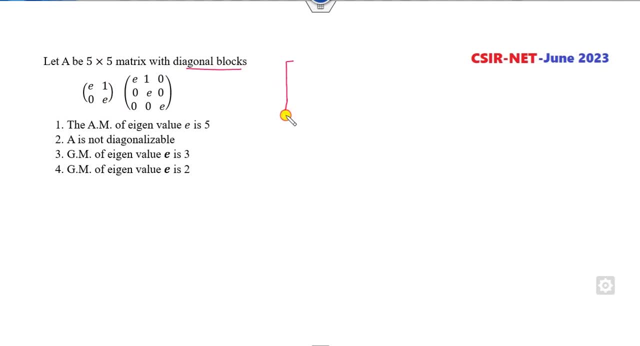 5 cross 5.. This is a diagonal block is given to you. So, firstly, it is a 5 cross 5.. And these are my diagonal blocks, So I can return this as a diagonal block here. This is the first. 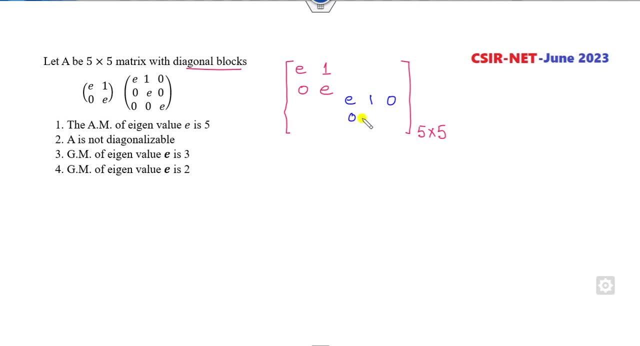 diagonal block. Second diagonal block is written from here: 0, e, 0, 0, 0, e. Rest values are my 0, 0.. Then which of the following is my correct statement? So look at that first. What is the? 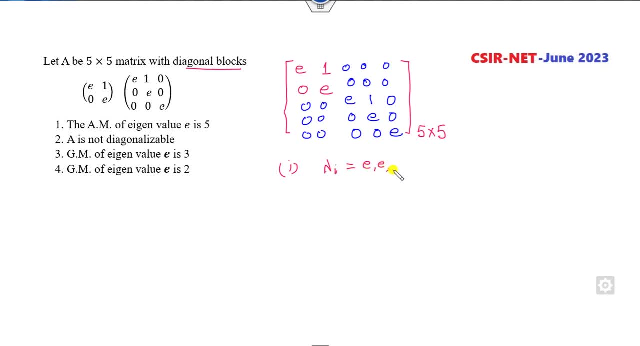 eigenvalues. So eigenvalues are my e. e how many times? 5 times. So arithmetic algebraic multiplicity of d lambda is my 5.. The first option is correct. one A is not diagonal. So how you can. 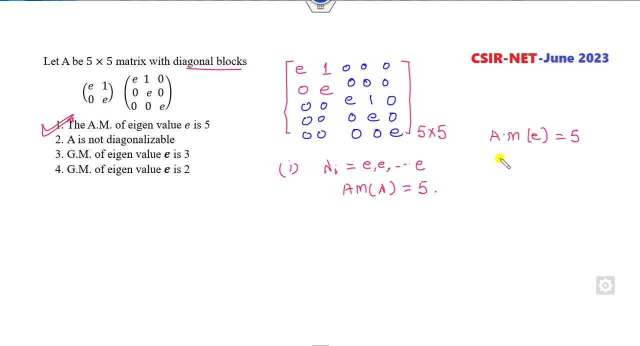 check that You have to find, the algebraic multiplicity of e is 5.. If we are able to find the geometric multiplicity of e, if this is not the algebraic multiplicity of e, then we have to not equal to 5. Then we can say it is not diagonal. Otherwise it is a diagonal. How you? 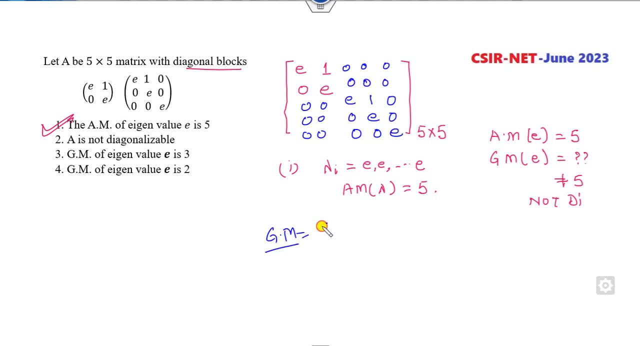 can find the geometric multiplicity. There are two methods. We already know This is a 5 cross 5, 5 minus rank of a minus e i. But here this is not the a, This is my diagonal matrix, So 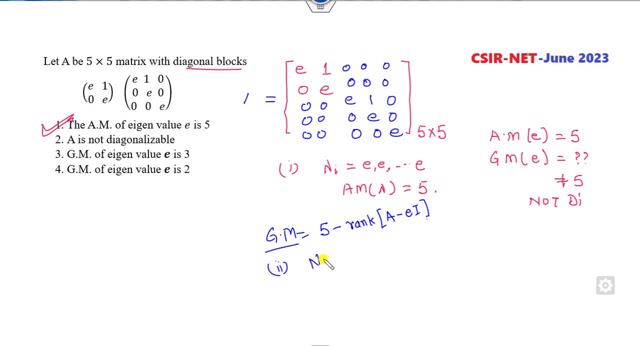 how you can find that. The second method is the number of the Jordan block. The number of the Jordan block is corresponding to the eigenvalue, is equal to the geometric multiplicity. There is a simple rule about that. Now you can count the number of the Jordan block. So this is the first Jordan block. This is the second Jordan block, This is the third Jordan block. So how many Jordan blocks are there? That is 3.. So geometric multiplicity is my 3.. So 2 is a cancel. So, since geometric multiplicity is 3, which is not equal to 5. So it is not a diagonal is also the 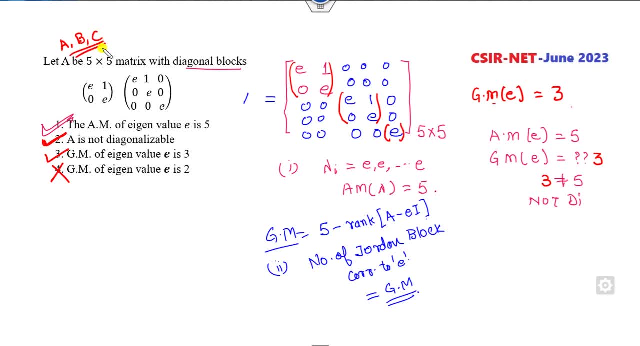 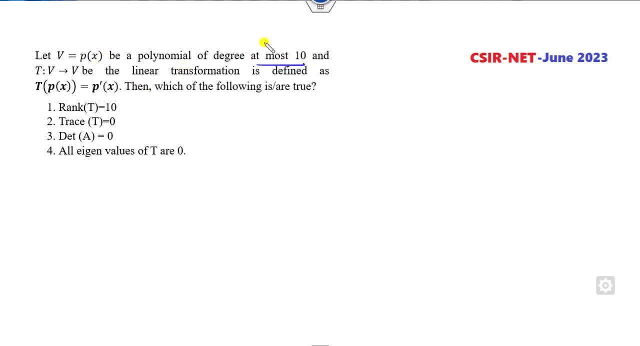 correct option. So a, b and c are my correct option of this example. Okay, look at this one. P is a polynomial of degree at most 10.. This is there. So the dimension of v is my n plus 1.. 10 plus 1 is 11.. You can see again the same formula: n, number of the variable, is my 1.. So you can see a polynomial of degree x. So it will be number of n. 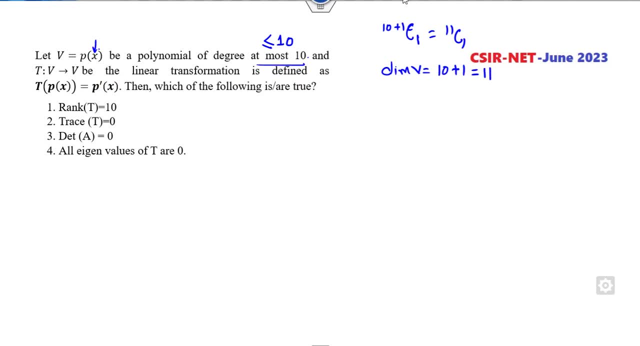 c 1.. 11 c 1 is 11.. A mapping is given to you as of here, So we can define 11 cross, 11 matrix. So what are the basis of this? 1, x, x, square, x, cube, up to x, 9 and x 10.. So what is that? Mapping is given to you as derivative. That is a very simple. So look at the first basis. If I consider p as 1, derivative will be 0.. That is a. 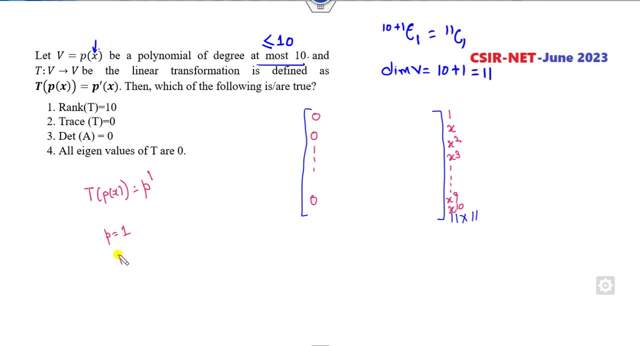 constant. Rest all values are my 0.. If I consider p as my x, the derivative will be my 1.. So corresponding to 1 is my here. Rest, all values are 0.. If I consider the polynomial as x square, basis x square, the derivative will be 2 x. The coefficient is my 2.. Rest values are my 0.. Similarly, if I consider x cube, derivative will be my 3 x square, So 3 x square is 3.. Rest values are my 0.. Similarly, if I consider x raised to power 10, derivative will be my 3 x square, So 3 x square is 3.. Rest values are my 0.. Similarly, if I consider x raised to power 10, derivative will be my 3 x square, So 3 x square is 3.. Rest values are my 0.. Similarly, if I consider x raised to power 10, derivative will be my 3 x square, So 3 x square is 3.. Rest values are my 0.. Similarly, if I consider x raised to power 10, derivative will be my 3 x square. So 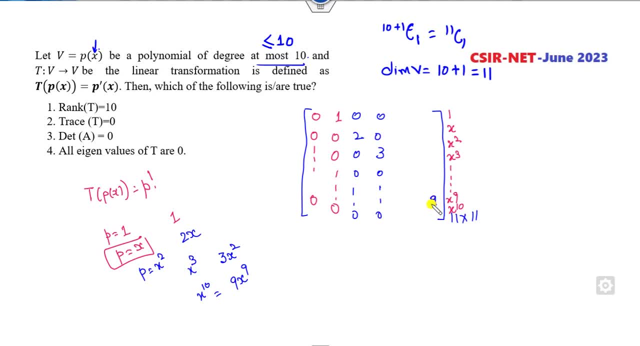 3 x square is 3.. Rest values are my 0.. Similarly, if I consider x raised to power 10, derivative will be my 3 x square. So 3 x value is nothing but my trace. so trace is also 10. determinant is also 0. all the eigenvalues are: 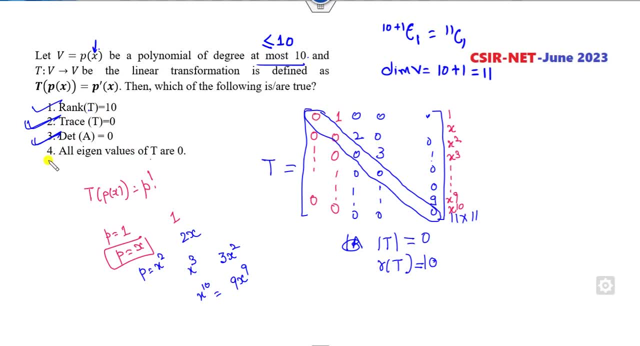 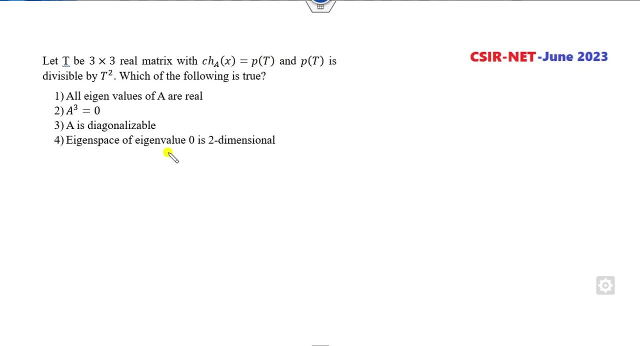 my 0 because it is a upper triangular matrix. so diagonal and trace are my eigenvalues. so all are my correct options of this example. okay, look at this one. t is my 3 cross 3 real matrix, such that characteristics polynomial is my p of t and p of t is divisible by t square. so what is the? 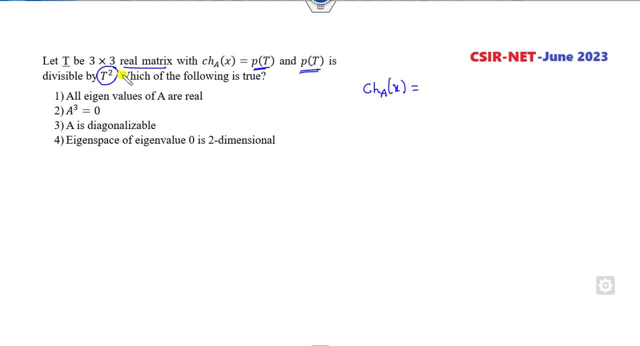 meaning of that the characteristics polynomial in terms of the x is divisible by t square, so definitely it will be x square of something then, only it will be divisible. now it's a 3 cross 3, so the two eigenvalue i have corresponding to this as a 0 comma 0. the third eigenvalue i can. 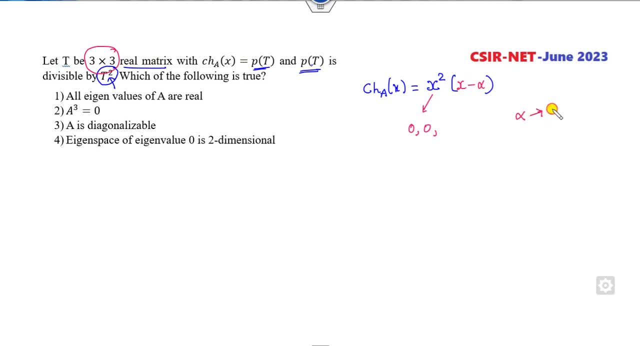 consider, say alpha. now this alpha may be the real or it may be a complex, but we all knows complex number. if alpha plus iota beta is my complex, is my eigenvalue, then alpha minus iota beta is also the complex value. but there is only one number. it means complex number will not be there, it means the. 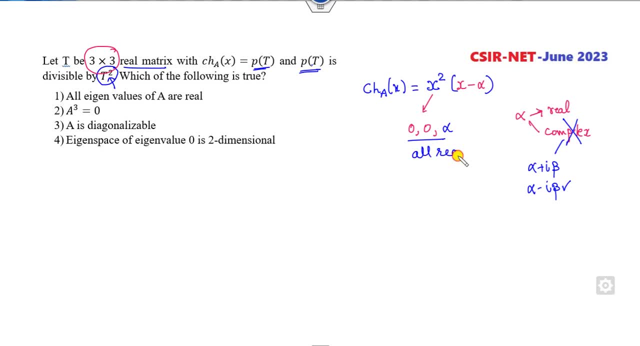 third eigenvalue is alpha. all are my real, so all the eigenvalues of the a are real is the right. so what is that now? a cube is a 0, or all about that. so it means that 2 eigenvalue must be 0. third eigenvalue will be: 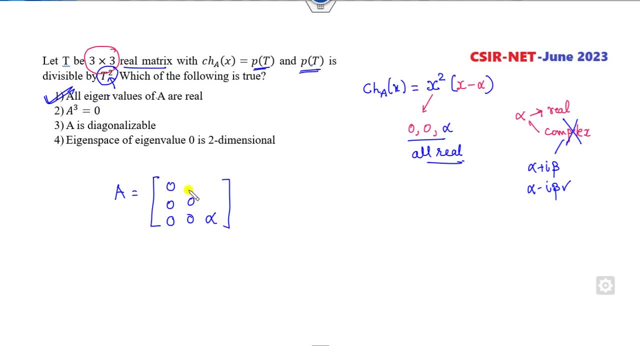 alpha. fine, so if i consider this is my a, for example, then what is the a cube? you can see easily if what is the eigenvalue of the a eigenvalue of the a are 0, 0 alpha eigenvalue of a cube is my 0, 0 alpha cube. so i can say what is the a cube? clearly say that all the values are 0. 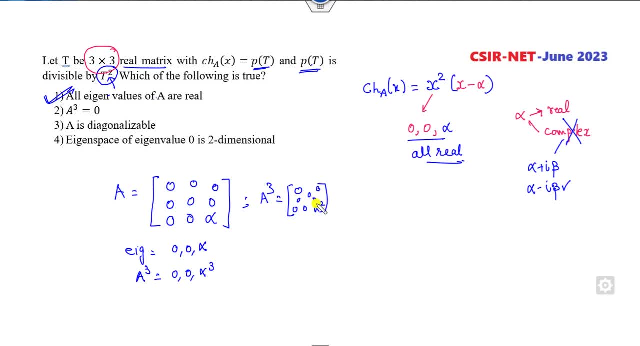 non-zero. fine, so clearly, say that which is, which is my, this is my non-zero, which is nothing but a. or say alpha square, which is nothing but is non-zero, because alpha is my non-zero. so it's alpha cube is a zero, is a wrong state, alpha is a diagonal. how you can see that? so what is the? 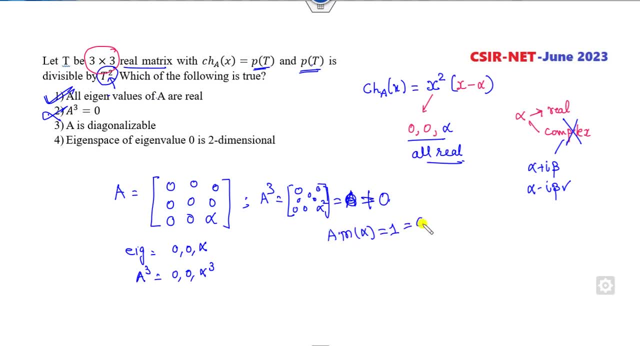 algebraic multiplicity of the alpha is a one, so, which is same as that of the geometric multiplicity. what is the algebraic multiplicity of the zero two? now you need to find the geometric multiplicity of the zero. if it is also that two, then it's a geometric, it's a, it's a diagonal. now, if i consider 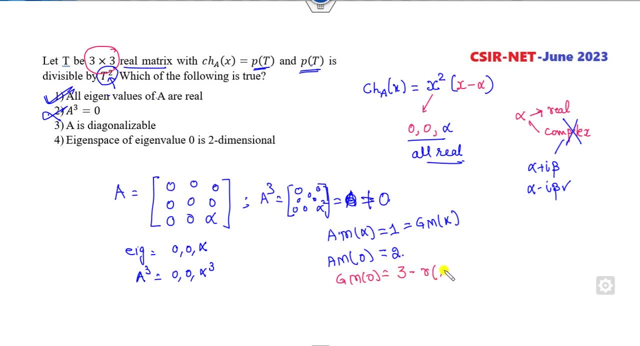 here it is three minus. rank of a minus zero: i. so if i consider this matrix, what is the rank of this? it's a one. so three minus one is a two, so they are same. but this is only one particular example. if i consider this number as say, my two, for example, then what is the rank of the a minus two i? there are the. 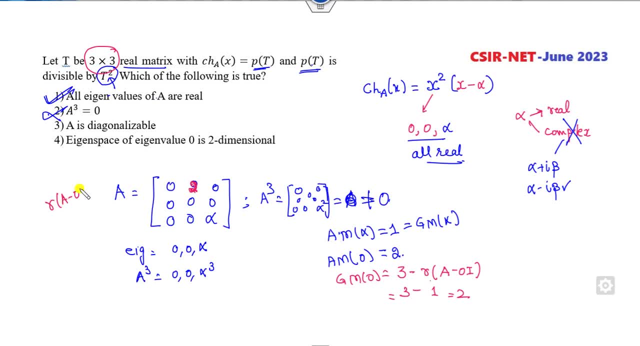 two non-zero rows, then the rank of a minus zero i is my one, because there are the one. sorry, the rank will be my two. so then three minus two, then the geometric multiplicity of this zero is my one, which is not equal to two. if i just simply consider this example again, the eigenvalues are zero. zero alpha is here, moreover, 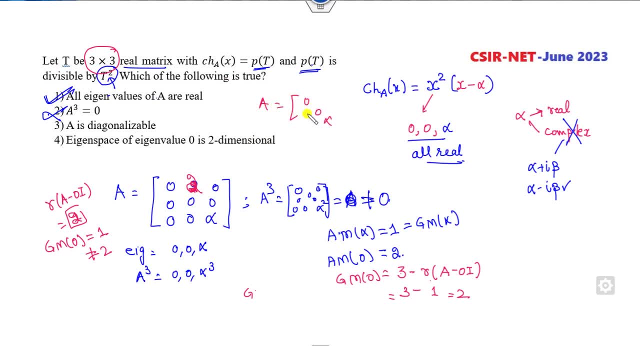 if you consider simply this example: zero, zero, alpha, zero, zero, say a, b and c, then clearly says that the rank will be my two and geometric multiplicity is not equal to two. so a is not diagonal is a wrong answer. eigen space, that is, a geometric multiplicity of zero, is my two. but look. 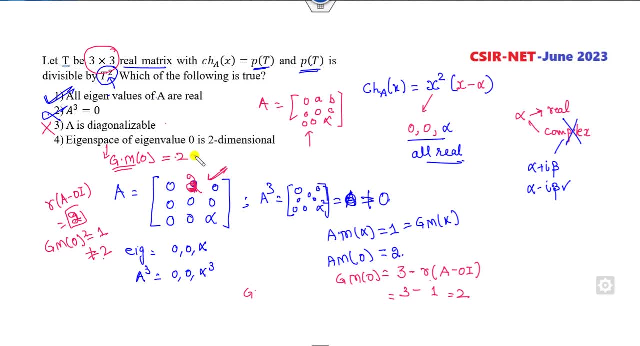 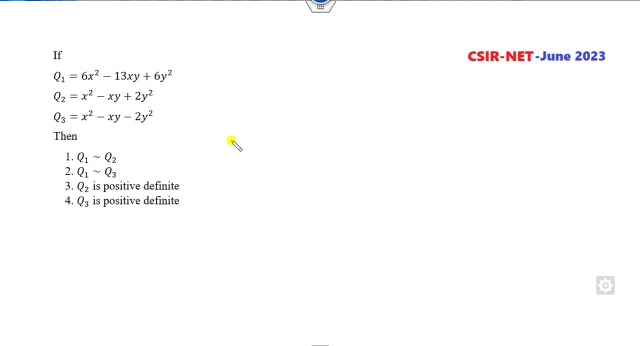 i consider this example, or this example is not equal to two because it is a. one which is not equal to two is also the cancel right option is only my. a is the correct answer. okay, which of the following is my equivalent positive, definite and here, so very simple. 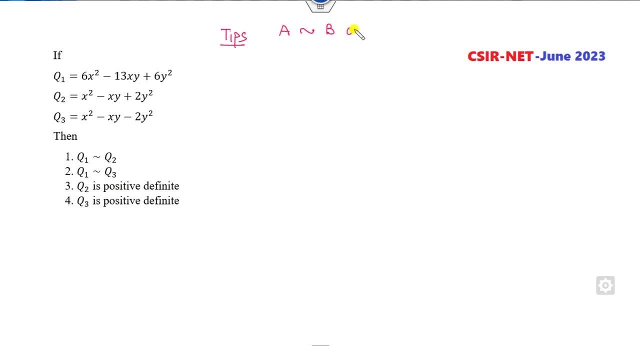 we can say: a matrix is equivalent to b over the r when rank of the a and rank of the b are same. second property: signature of the a and signature of the b are same. what is the signature? is the difference between the positive eigenvalue and the negative eigenvalue. now we can define over. 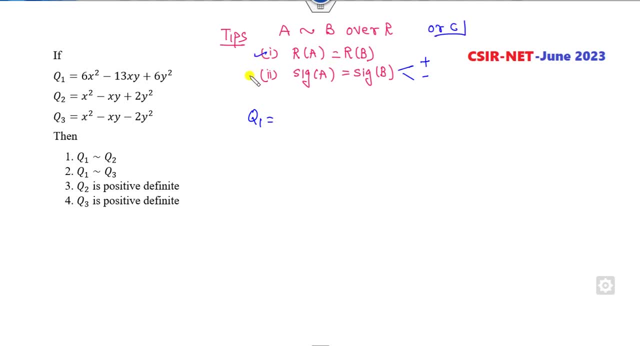 if it is over the r, then these are the two properties. if it is over the c, then only the first property is enough to prove that equivalent. now you can write the equivalent matrix of the k1. diagonal values are my 6 and 6, half of this: 13 minus 13 by 2 minus 13 by 2. look at the k2. 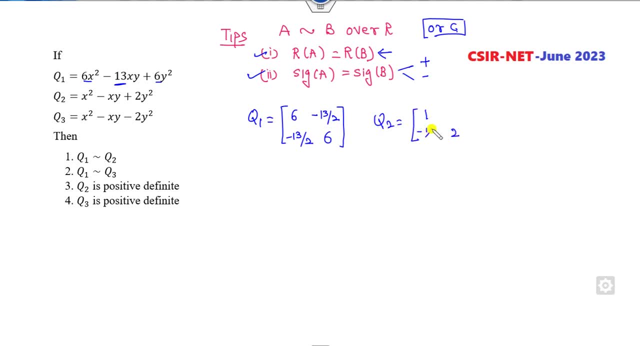 what is that k2? 1, 2, half of the coefficient of the x- y. this is my. what is the k3? 1 minus 2 minus half, minus up. now we can find the rank of this. clearly say that determinant of the k1 is: 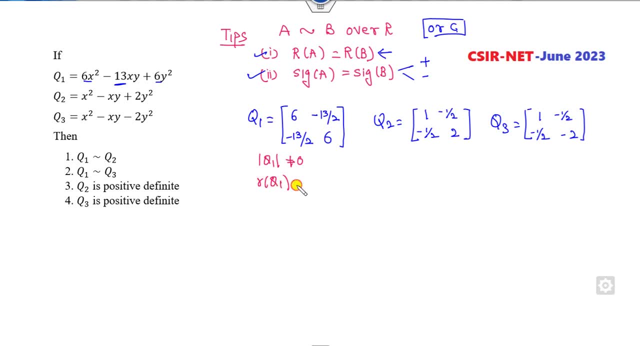 non-zero, 36 minus this. so what is the meaning of that? rank of k1 is my 2. determinant of the k2 is 2 minus 1 by 4, again a non-zero. so the rank of k2 is my 2. determinant of k3 is again a non-zero. so the rank of the k3 is my 2, the first property. 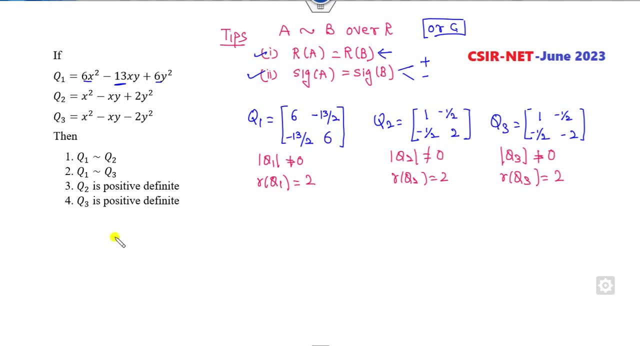 satisfied in all case. now we can find the eigenvalues. how you can find the eigenvalue? we can check about the principal minus. the first principal minor is 6, which is greater than 0. second principal minor is the determinant 36 minus 169 over 4, which is less than 0. what is the meaning of that? it is negative, definite. 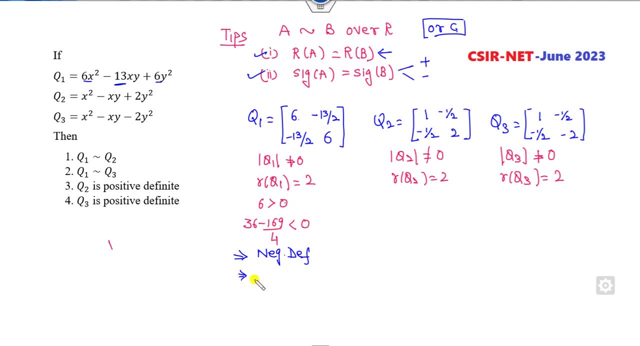 because the first principal minor is positive, second is negative. what is the meaning of that? one eigenvalue is positive, second eigenvalue is negative. look at this: the first principal minor is 1, which is a greater than equal to 0. second is 2 minus 1 by 4, which is again a greater. 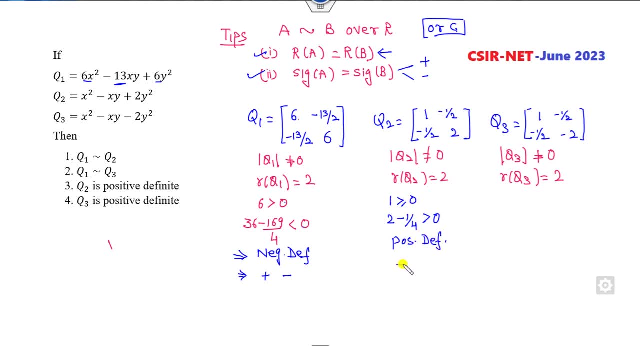 than 0. it means it is my positive definite: the both eigenvalues are my positive. first, principal minus greater than 0. second is my minus 2 minus 1 by 4 less than 0. it is a negative definite. one eigenvalue is positive, second eigenvalue is negative. so what is my signature? 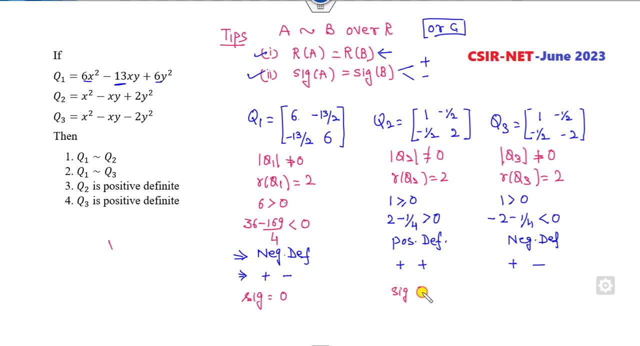 1: 1: 0. signature is 2. there is no negative root. what is the? signature is 0, so signature 0, signature 0. rank: both are same. k1 and k3 are equivalent. the first option is cancelled. 3 are positive definite, only q. 2 is my positive definite, so the right answer is my. b and c are the 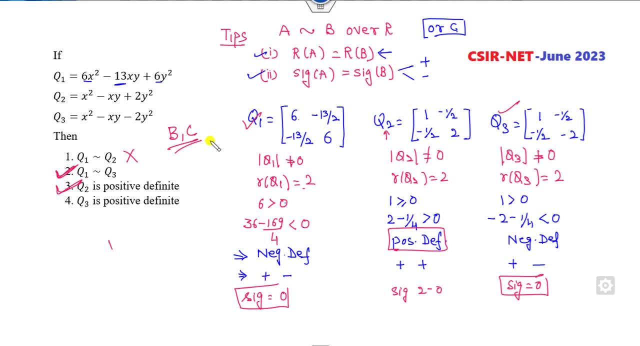 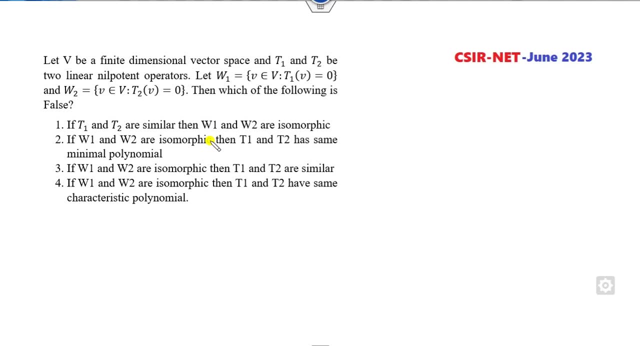 right answers, very simple, elementary questions. they are asked in this june 2023 linear algebra. okay, look at this. another one again. this is a very simple question. v is a finite dimension vector, space. p 1 and t 2 are my nilpotent matrix, such that v 1 is here, v 2 is this then, which of? 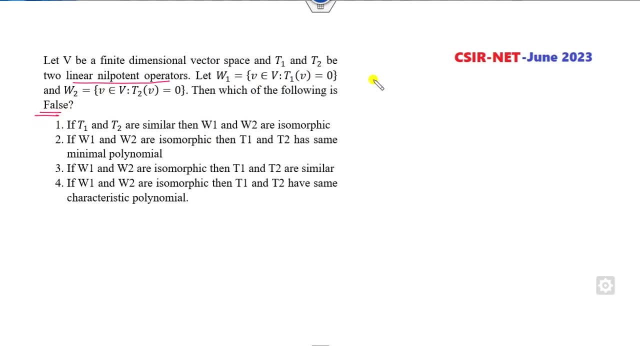 the following statement is my false statement. fine, t 1 is similar to t 2. what is the meaning of that characteristics polynomial of t 1 is same as that of the characteristics polynomial of this, or you can say: the minimal polynomial of this. minimal polynomial of t 1 is same as that of: 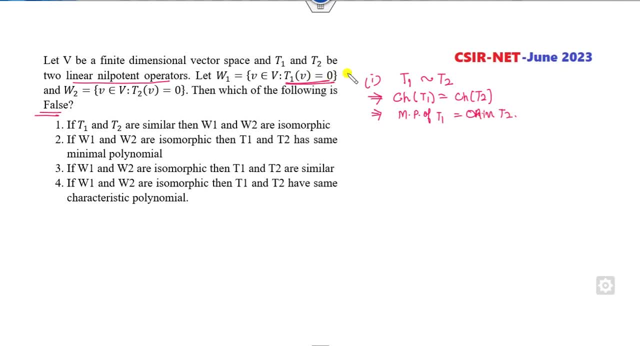 the minimal polynomial of t 2. now you can see what is that this is represent, about the nullity. so we can say: what is the minimal polynomial? minimal polynomial always represents about the geometric multiplicity of geometric multiplicity of the eigenvalue. fine, what is the? 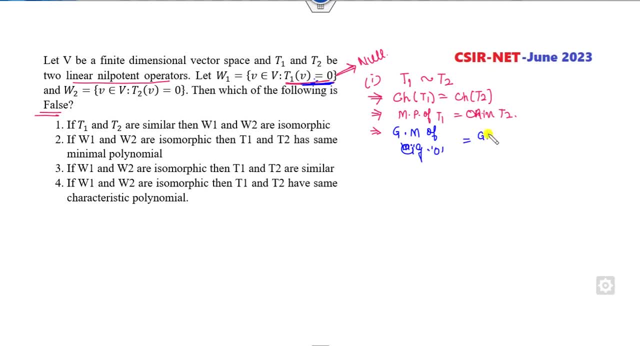 eigenvalue of this is a 0, so it means geometric multiplicity of the eigenvalue 0 in the t 2 are same. what is the meaning of that? nullity of t 1 is nullity of t 2. what is the meaning of that? 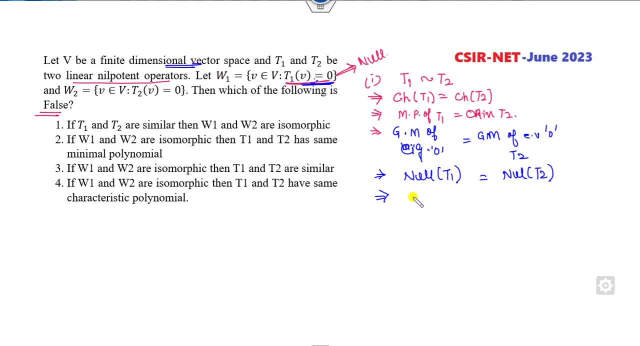 once nullity are same, there is a finite dimension, so rank will be finite. you can see that dimension of t 1, that is a w 1, is same as that of w 2. what is the meaning of that? once both are dimensions same and they are finite dimension, it means they are isomorphic to each other. the first option is my. 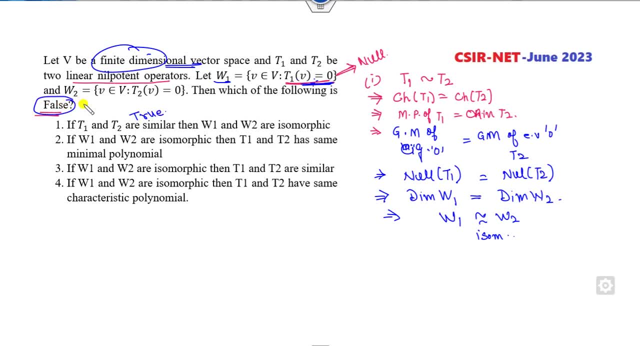 correct statement, but we need a false state. look at the second part. if w 1 and w 2 are isomorphic, what is the meaning of this? if w 1 is isomorphic, then what is the meaning of this if w 2 is isomorphic? 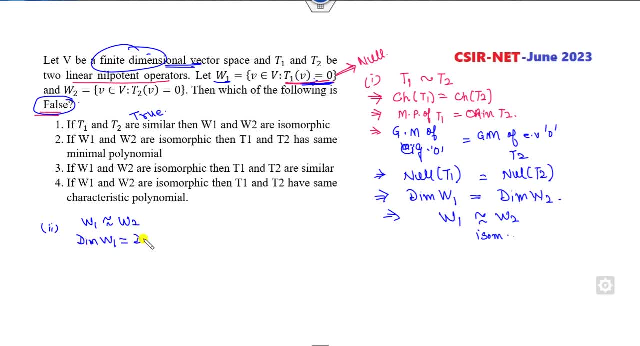 that dimension of w1 is same as that of dimension of w2. fine, done, are the same. minimal polynomial. how you can think about the minimal polynomial, either you can define the characteristics polynomial or you can define the number of the jordan blocks. that's the same thing for here. 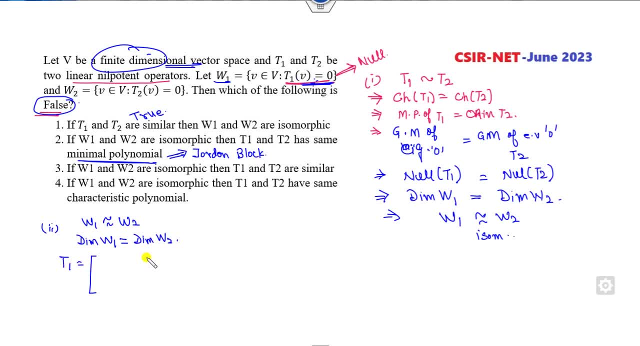 now, if i consider that two example here, like first example, i can, since here zero, zero, one, zero, say here fine. and second is similar to this: i just interchange my row here: zero, zero, one, zero, zero, zero, zero, zero, fine. or i can more simplify. i can simply take: this is zero and this is my. 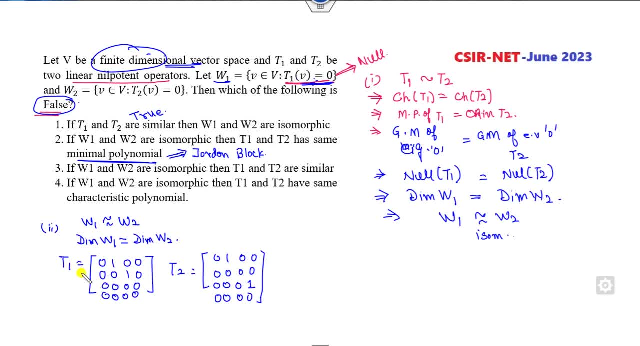 one. then what is that dimension of this? it's a four cross four. rank is my two. nullity of t1 is my two. nullity of t2 is also my two. rank is also two. rank is also two. it means the dimension is my same. it's satisfied. now, nullity are same. does it implies the minimal polynomial? that is not always. 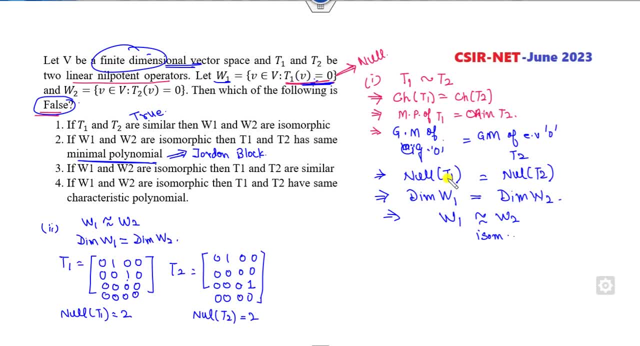 two, converse is two. if minimal polynomials are same, nullity are same. but look at that. how many jordan blocks are there? one, two, so it means their minimal polynomial is lambda square. there are two jordan blocks. look at that. one, two, three. the minimal polynomial of this is my q, so it means the minimal polynomial. 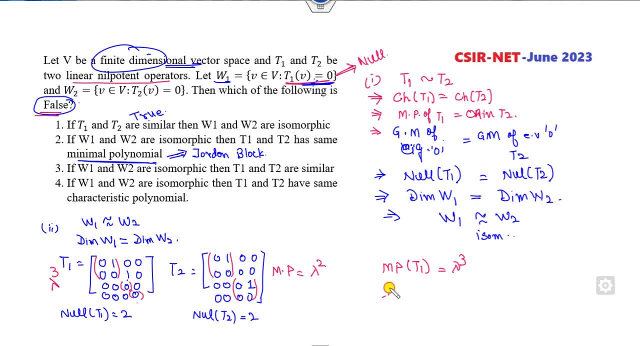 of t1 is my here, which is not same as that of the minimal polynomial of this. so second option is false. thus, if second option is a false, it means this is my correct option. if w1 and w2 are isomorphic, there's the same examples. then t1 and t2 are similar to each other. so if w1 and w2 are isomorphic, 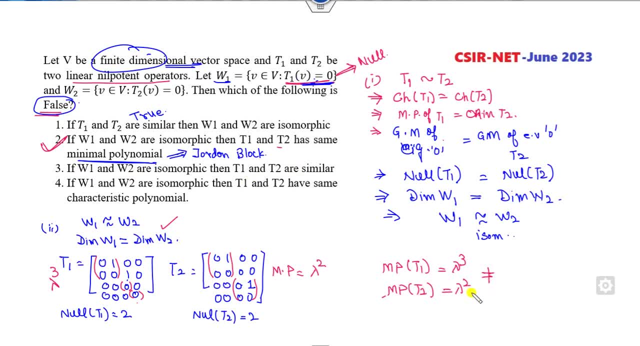 again. you can see minimal polynomials are not same. it means they are not similar to them, they are not isomorphic of them. it means t1 is not isomorphic to t2. that means they are not similar. so this option is also false. so this is the correct state if w1 and w2 are isomorphic. again the same example. 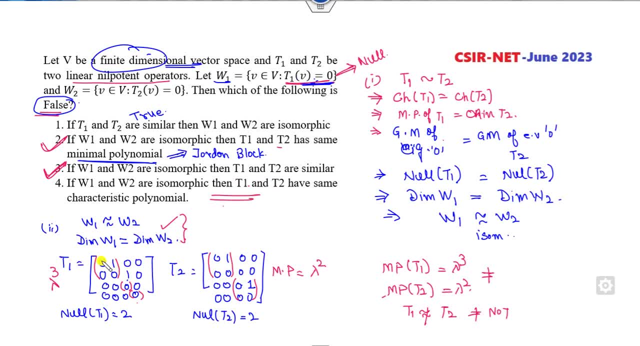 then they have the same characters. there's a simple result because you can see the characteristics polynomial of this is lambda, 4, r4 and or more more of the same example. if w1 and w2 are isomorphic, however, this is the standard result. if w1 is isomorphic to w2, the corresponding characteristics. 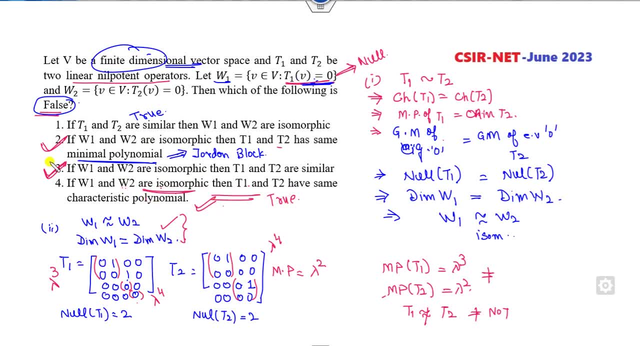 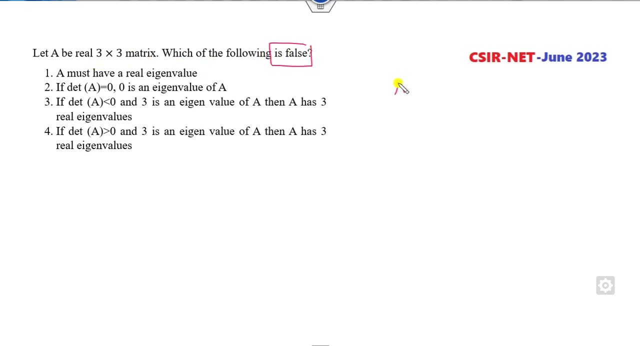 polynomial are always same. so this is my true statement. this is my false statement. this is my false. so right answers are my b and c are the correct option of this example. okay, look at that. a is my 3 cross 3 real matrix, which are a falling statement is my false. so this is my 3 cross 3. 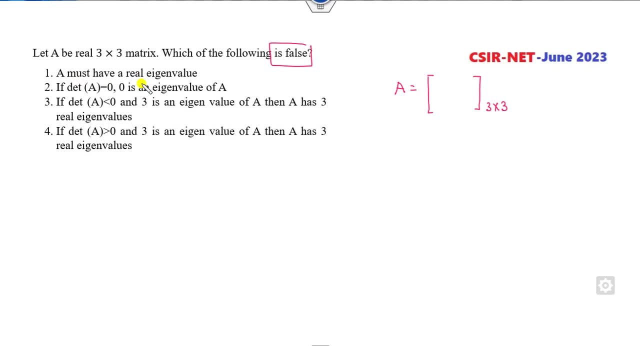 then the first option is: a must have a real eigenvalue. a must have a real eigenvalue. okay. so if you find the characteristics polynomial of a, it will be a cubic equation. fine. and we all knows, a polynomial having the odd, odd degree polynomial must have at least, must have at least one real root. that's the simple. 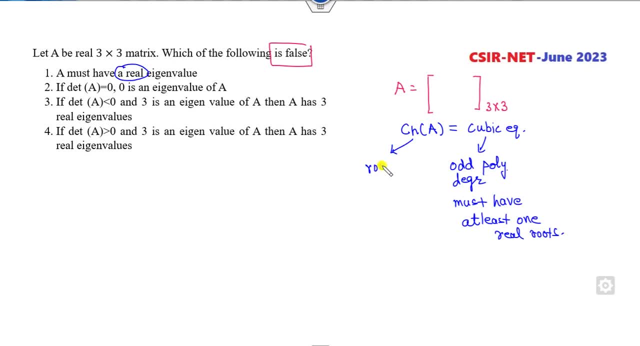 property we all knows. now the characteristics polynomial has the root. what is the root of the characteristics polynomial? that is the eigenvalue. so, since it is a cubic polynomial, so that it must have a at least one real eigenvalue. this statement is my true statement. but we need a false state. if determinant is a 0, then 0 is the eigenvalue. that's a obvious. 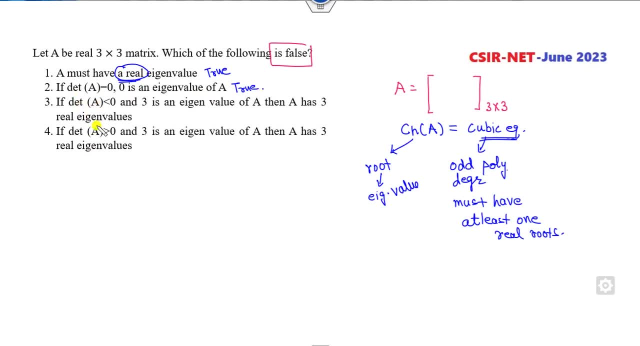 statement. it's the correct statement. if determinant is my negative and 3 is my eigenvalue, there are the three eigenvalues. if 3 is my eigenvalue, then a is my real eigenvalue and b is my real eigenvalue. okay. so if i consider, this is my complex number, say alpha plus iota, beta, this is also the complex. 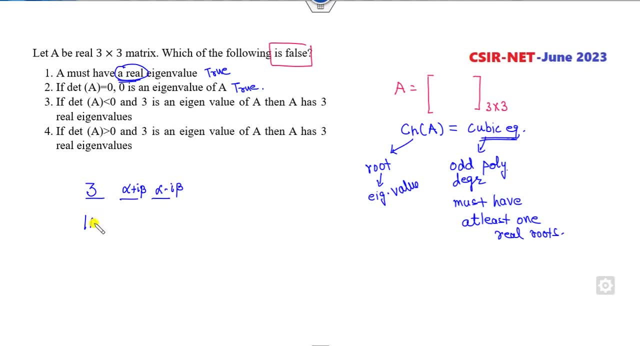 number because they are occurring, the pair. what is the determinant of this matrix? 3, alpha square plus beta square, which is greater than 0. so, but we need a less than 0. so you can see. so whenever determinant is less than 0, it means none of the values are complex, it means both the values are. 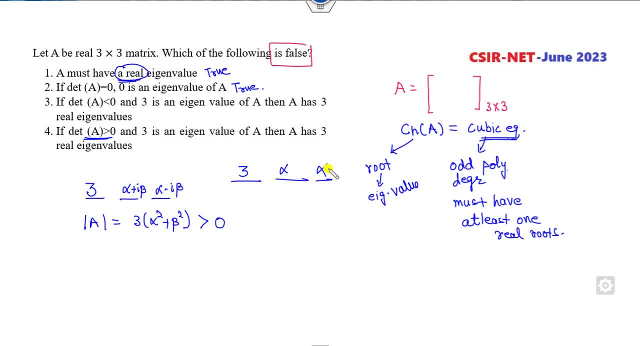 real. so then both the values are real. so then both the values are real. so then both the values are real. it may be alpha 1 and alpha 2, then the product has at least the three eigenvalues. that's the correct statement. both all are my real eigenvalue. this is the correct state, the only left. 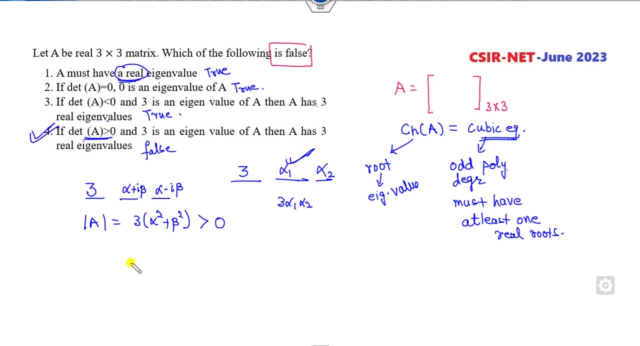 option is there which is my false. that is the right answer and this is the explanation of this. if determinant is my positive, then a has a three real eigenvalue. that's not true. yeah, i can simply take. if one eigenvalue is iota, other eigenvalues minus iota, then what is the 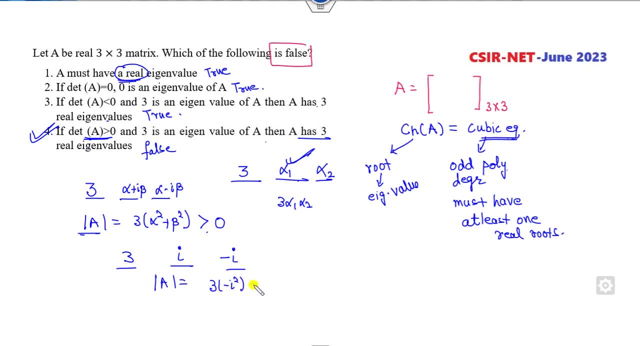 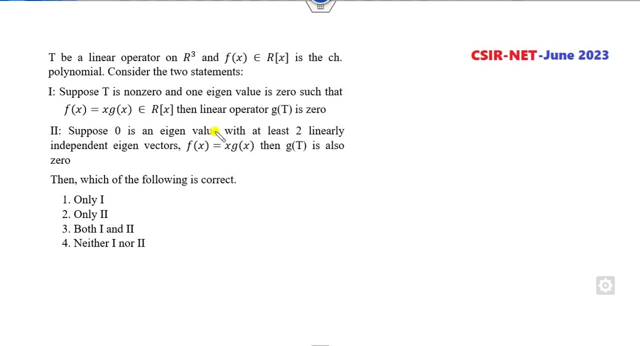 determinant of this three minus iota square is my three, which is greater than zero, but eigenvalues are my complex number as well. so the right answer is my four, which is actually the false state. okay, look at this. another one: t is my linear operator, f is my. here. consider that two, statement one and two, which are 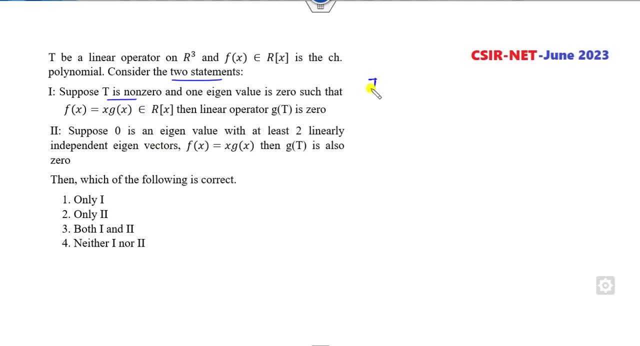 the following is the correct. okay, look at the first statement. t is my non-zero and one eigenvalue is my zero. it's a r cube. so t is my three cross, three matrix. one eigenvalue is my zero. what are the other eigenvalues? if i consider alpha 1 and alpha 2? okay, then what is the characteristics polynomial? 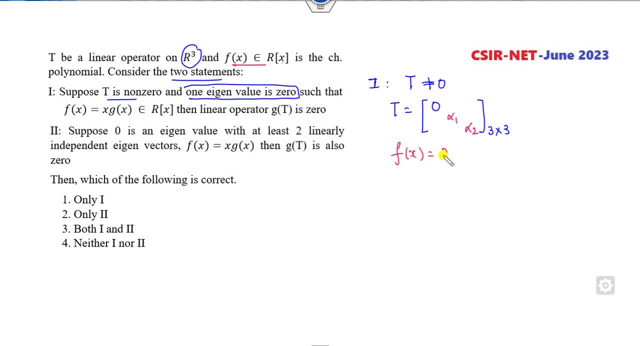 of this. fx is my here. so what is that? i can return as x. x minus alpha 1, x minus alpha 2. alpha 1 may equal to alpha 2 or it may not equal to alpha 2. then fx is my here. then g of t. so what is the my g of x? this is my g of x, if i compare this with here. 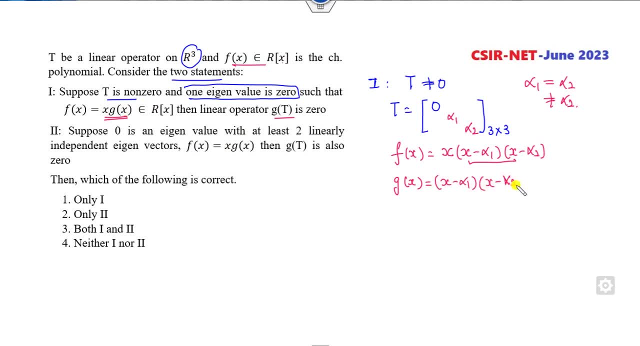 so x minus alpha 1, x minus alpha 2. fine, then our target is to prove g of t is my zero. this is we need to check. very simple: if i simply consider alpha 1 and alpha 2, both are same, say four, or you can see any of the number. i can say one, a simple one. so or? 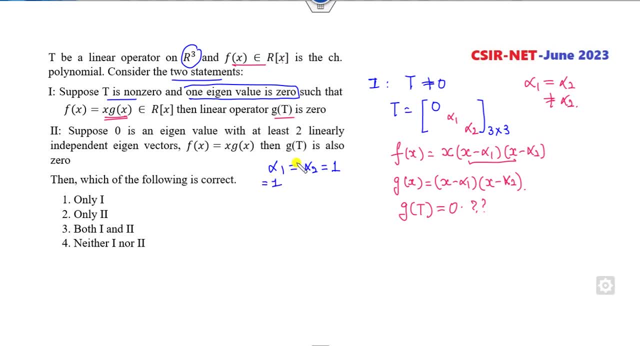 this is a Ruby rupee, easily 19, 2. this is my minus of 2, so it is my. of this a square. this is x minus 2. this is x plus 2, x square minus 4. fine, so that its coefficient is not same. now, what is my actual value of the t? 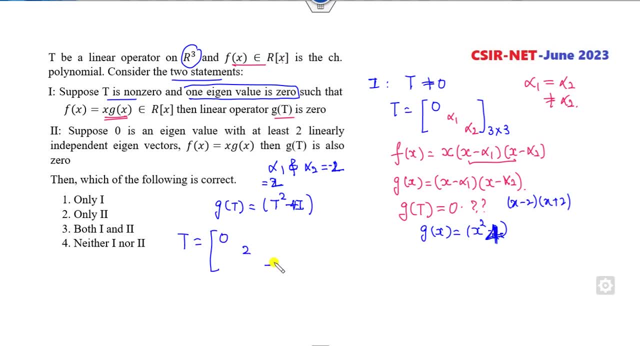 one eigenvalue is 0, other eigenvalue is my 2 and third is my minus of fine, if i consider this simple matrix, then what is my t square? what is the eigenvalue? 0, 2 minus 2? are the eigenvalues of the a. what is the eigenvalue of the t square? 0, 4, 4, fine. what is the eigenvalue of the 4 i? 0, 4, 4, 4. 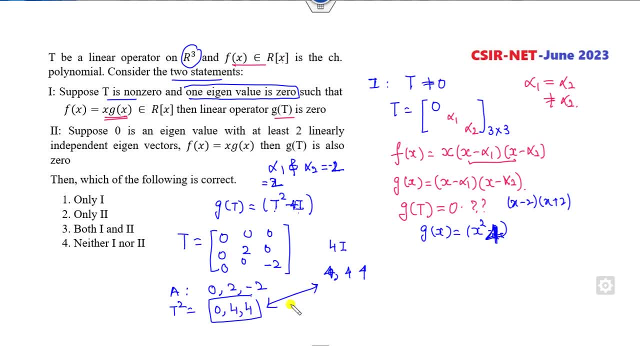 if i subtract them, what is the eigenvalue of their subtraction? it will be 4 0, 0. it means g of t could be like of this 4 0, 0 below and clearly say that this is not my 0 matrix. so but he said it's. 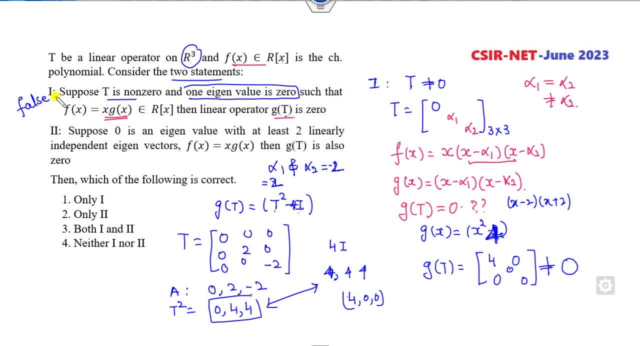 0 is my 0 false state. i hope you can easily understand that you can consider any of the alpha 1 and alpha 2 i can simply take for this simply calculation. you may consider this as alpha 1 and alpha 2 as here, like if i solve for you. if i simply take: alpha 1 is 1, alpha 2 is my minus 1, then this number will. 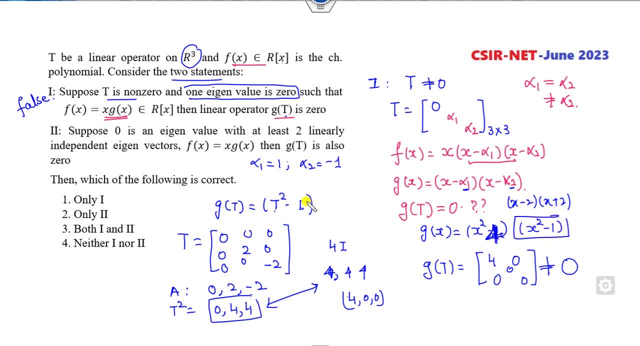 be x square minus 1. so g is my x square minus 1. so this number will be my: 1 minus 1 eigenvalue will be 0, 1 minus 1. eigenvalue of that t square will be 0: 1, 1. eigenvalue of the i will be 1 1, 1 if you. 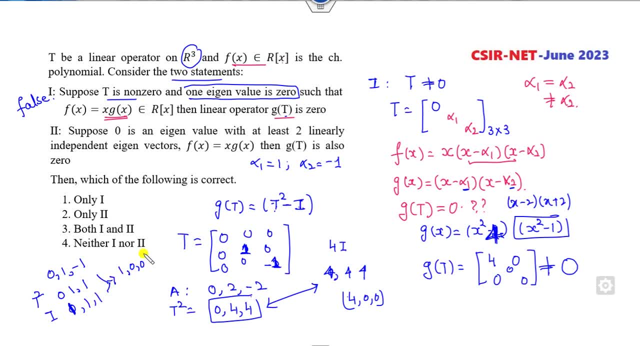 subtract them. what are eigenvalues? 1 0 0. so if this matrix has the eigenvalue 1 0 0, it means 1 0 0. so if this matrix has the eigenvalue 1 0 0, it means 1 0 0. so if this matrix has the eigenvalue: 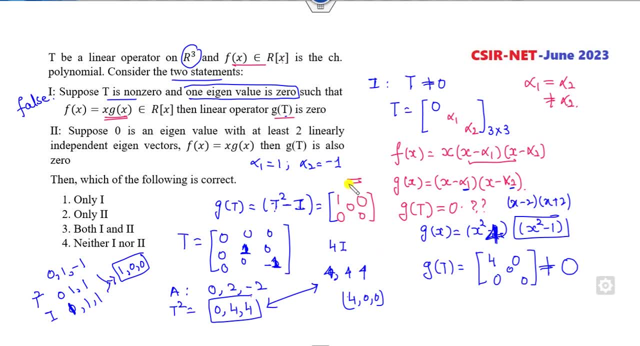 the matrix could be like of this nature, which is clearly say that it's a non-g. fine, now look at the second study. what is the second study, said you suppose 0 is eigenvalue with at least 2 linearly independent eigenvector. what is the at least 2 eigenvalue? that's a geometric multiplicity, is my. 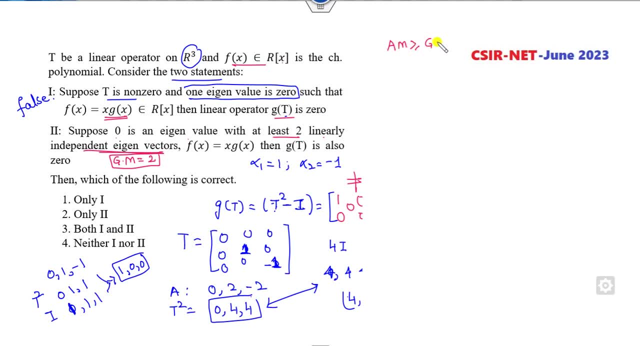 2 and we all knows algebraic multiplicity is greater than equal to here. so it means algebraic multiplicity can be 2 or 3. so firstly i consider the case of the 2. it means 2 occurring eigenvalues are my 2. the third: 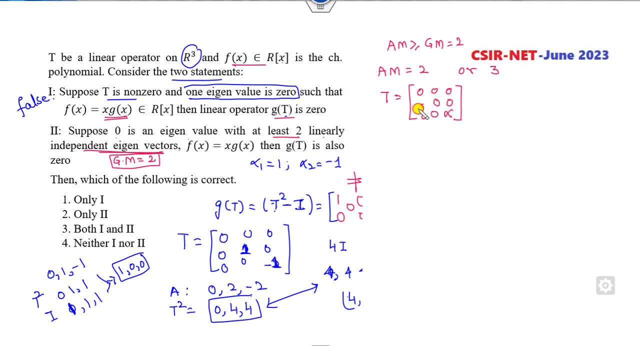 eigenvalue i consider as a 0. then according to this, what is that? it is my x square x minus alpha. then what is the g of x? if i consider from here, this is x into x minus alpha, or i can return as x square minus alpha x, then what is my g of t? 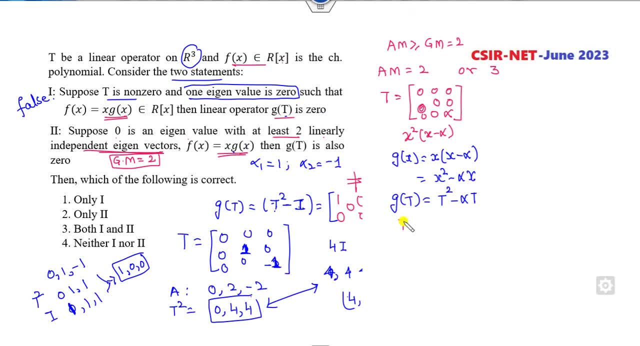 square minus alpha of t. fine, so what is the eigenvalue of that? t is 0, 0 alpha. eigenvalue of that t square is 0, 0 alpha square. eigenvalue of the alpha into t is 0, 0 alpha square. fine, whatever the value of the alpha. now you need a subtract. if i found the eigenvalue of that t. 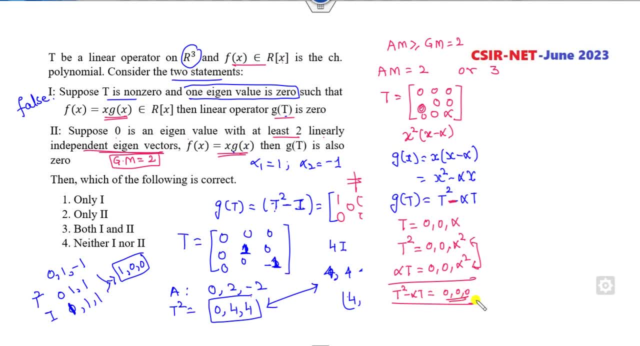 square minus alpha t, it is my 0 0 0. so it means this value will be my here. so it means this: this matrix must be a 0 matrix. if I consider all the eigenvalues are 0, what is the meaning of that? this is my nilpotent matrix, and what is that? this is the x cube. so if this is a, 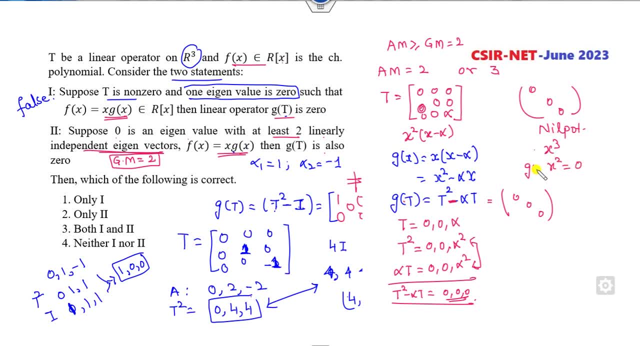 nilpotent matrix. so x square will also be a 0, because this is my gx in this case, as compared to this, so in this case it is also be a 0, so it means this is my correct state. so, once this is the correct statement, so only 2 is my correct statement, is the right answer. 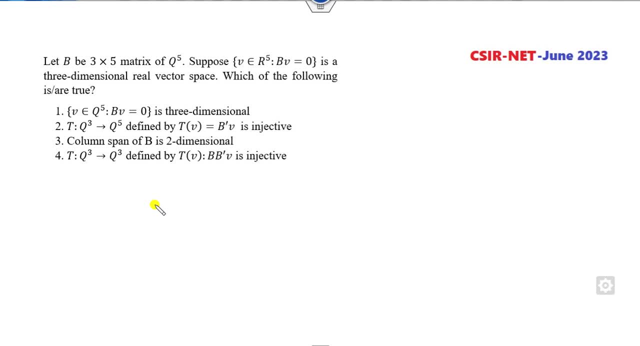 of this exam. okay, look at this another one. b is my 3 cross 5, such that this: what is that? this is nothing, but my ax is 0. or you can say this is a nullity of a because 0 is a 3 dimension vector. so nullity of the nullity of b, that is a nullity of b is my 3, so can. 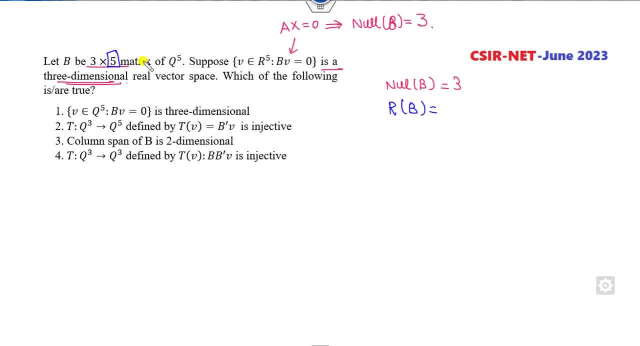 you find the rank of the vector b. what is that? this is a 5 number of the column vectors minus nullity of the b. so that is, the rank is my 2, rank is my 2. then, once the rank is my 2, the column span of the b is my. 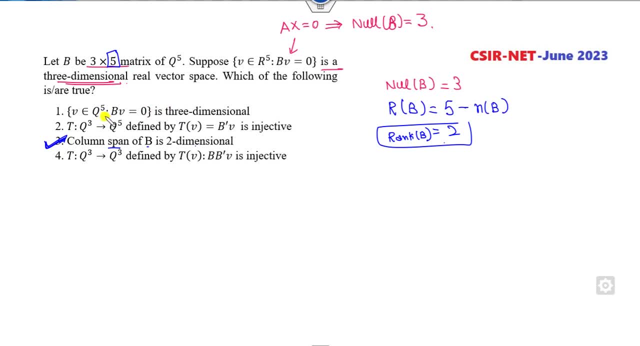 2 dimension is the correct state, then first option is okay. this is on the r cube. that means if you have the 3 cross 5 matrix elements are my real numbers. Now if the elements are from the q, what is happening on the matrix? nothing is there. that. 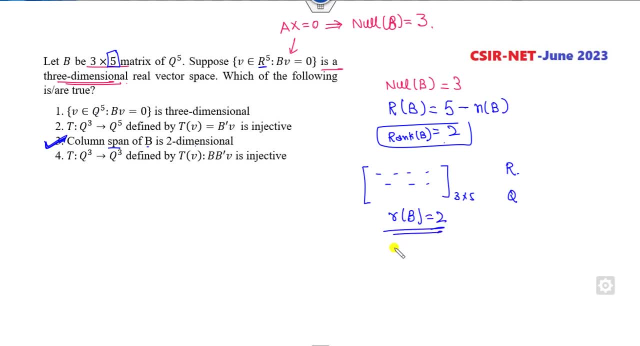 the rank will be the same. rank will be my same. that means nullity is my same. if rank is same, nullity is same. so this is again a 0. so they are talking about the nullity of the b. when vector is from the q, then again it is a. 3 dimension is the correct answer. 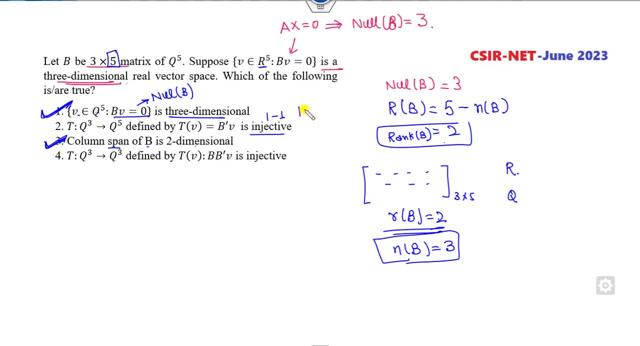 okay, then is a injective 1- 1. how you can prove that 1- 1?? if you prove that, if you prove that nullity of t is my 0, that means, if you prove that nullity of t is my 0, then it is a 1, 1. now it is a b transpose. what is the rank of the b transpose? we all. 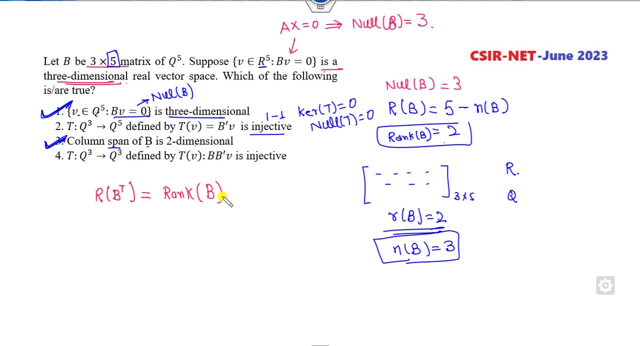 knows rank of the b and the rank of the b transpose. both are same. so this is my rank, is my 2, so this is my 2. and what is that? nullity of b transpose number of the dimensions are my 3, so 3 minus rank of the b transpose, it is my 1, which is non-zero. it means it is not. 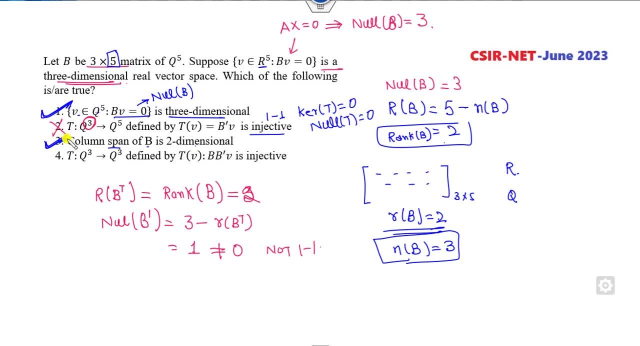 1- 1. so this option is cancelled. look at this one again. it is a: 1: 1. so you have to prove the kernel of this. t is my 0. it means your target is to prove nullity of b into b transpose is my 0. now we all knows what is the rank of the b into b transpose. it is the same as. 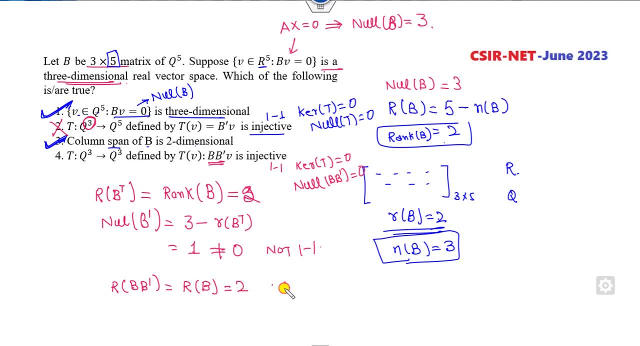 the rank of the b, which is again the 2. so what is the nullity of b into b transpose? so what is that? domain is 3 and minus rank of the b into b, which is 1, which is non-zero. so it is not a 1: 1, but he said a 1 1, so the right answer is a and c. are my correct options that? 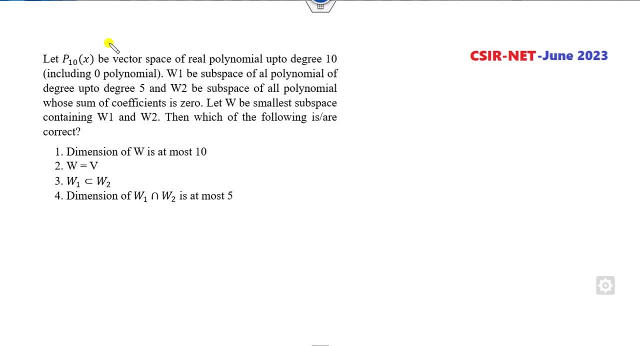 is a very simple, straightforward transport. okay, look at this next one. p 10 is a vector space of the degree 10, so what is the dimension of this? p of 10, 11, w 1 is a subspace of all the polynomial up to degree 5. so what is the dimension of w 1, 6, v, 2 is the subspace of. 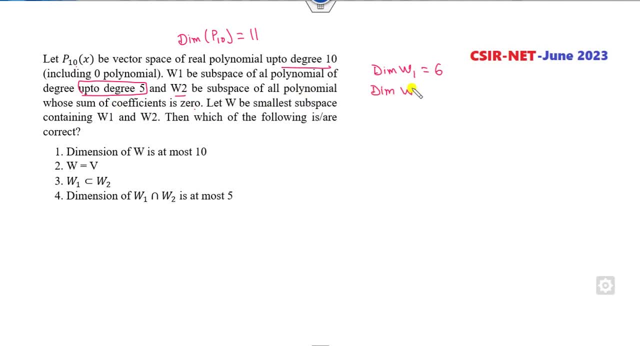 all the polynomials. w 2 is the subspace of all those polynomials from the p of 10, such that The coefficient is my 0. okay, and what is the p 1 is all those polynomials from the degree of p 5. this is my p, w 1 and w 2. so what is the dimension of this? dimension of this is: 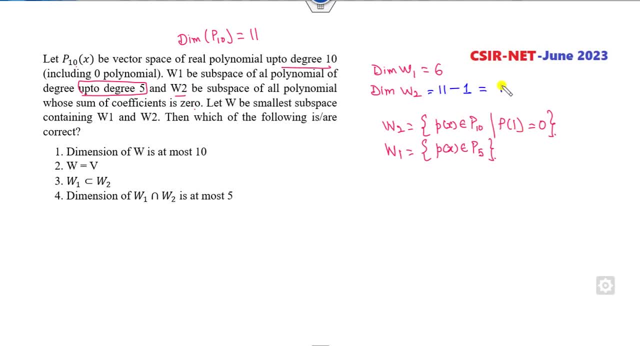 11. there is only one condition, so it is a minus 1, so it is my here. then w is my smallest subspace. of what is the smallest subspace is, we all knows, the smallest subspace is my w 1 plus w 2.. 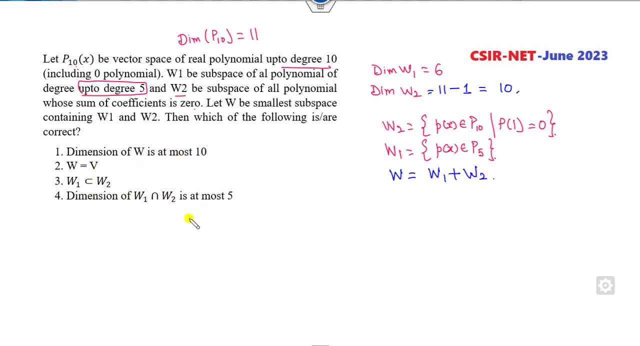 Then the dimension of this, Dimension of this, dimension of this and so on. very simple: firstly, we can see about here, if I consider any of the element from here, if I say x 4, this is my w 1, is it belongs to w 2? no, why? because the w 2 consists of all those subspaces, all those polynomial whose 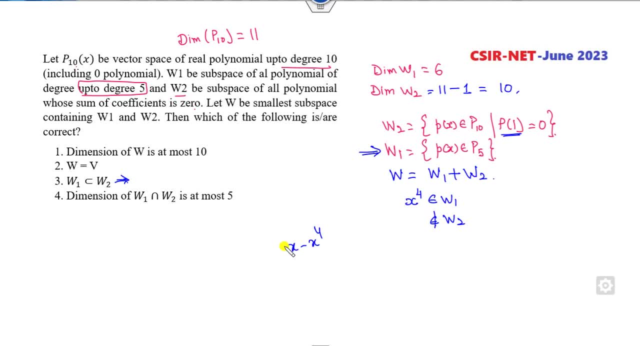 coefficient will be 0, like x minus x: 4. the coefficient is 1 minus 1, 0, but here the coefficient is 1, which is not 0. So it means W 1 does Not contain in the w 2. this option is cancel. 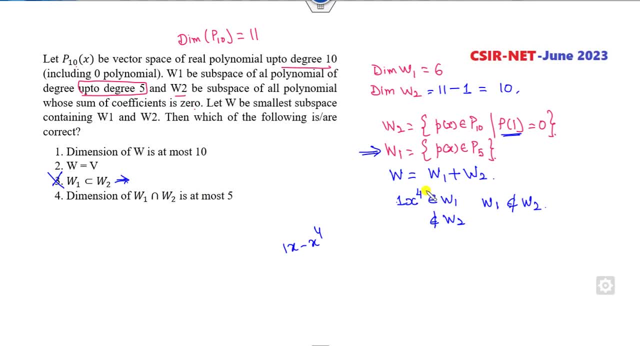 Now look at the intersection. what is the w? now we can check about this w. how you can check about? firstly, we can check about the dimension of w. so what is that? this is dimension of w 1. dimension of w 2 minus. dimension of w 1 plus w 2. so what is that? dimension of? 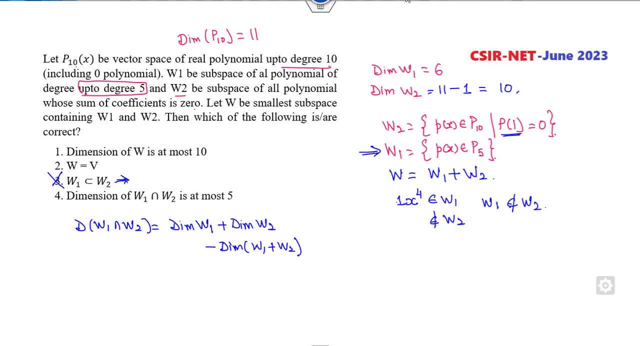 w 1 and w 2. is here, so we need to find it. so firstly, we will check about that, how you can check that. that is my here. so again, i think it's a very simple how you can think about that. if i think about here: what is the intersection of this collection of all those polynomials? 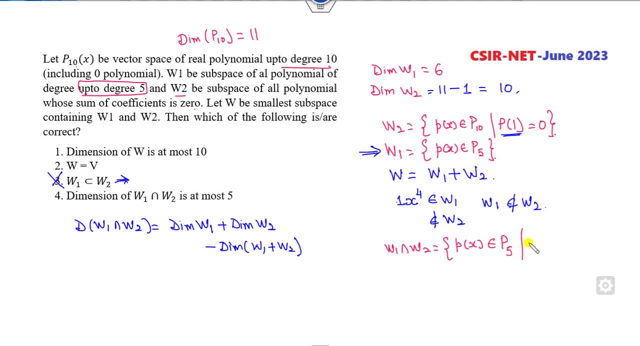 from the p5, because the intersection is p5, such that this is my here. fine, so what is the dimension of this? so what is the dimension of this? is 5. sorry, p5 is a sixth dimension. this is my 6. there is a 1 condition involved. so 6 minus 1 is my 5. so this is my 5. so dimension: 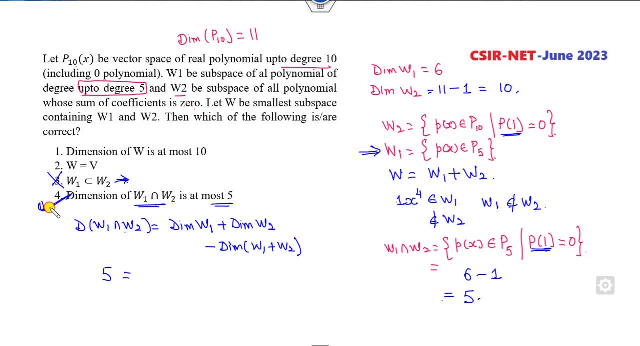 of dw1 is at most 5. this is 5. that's the correct, is the correct statement. so this is my 6, this is my 10 and this is my x. so what is that? it's a 16. so x will be my 11. what is the meaning of that? 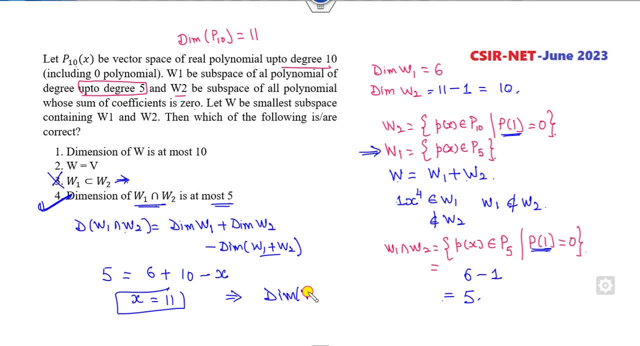 dimension of w1 plus w2 is nothing, but my w is my 11, so dimension of w is at most 10. that's a wrong state. now, w and v- this is my v vector space and both are my finite dimension. so, as i discussed in the previous example, if dimensions are same, you can see w and v are my same because 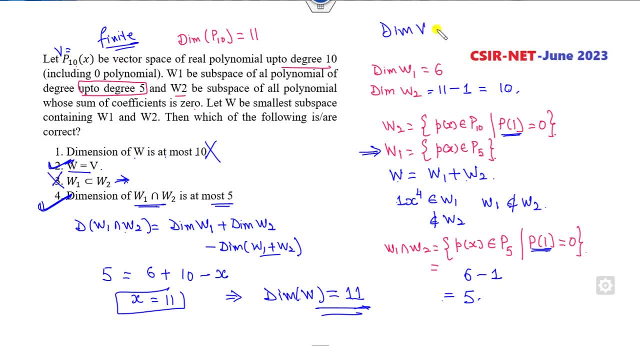 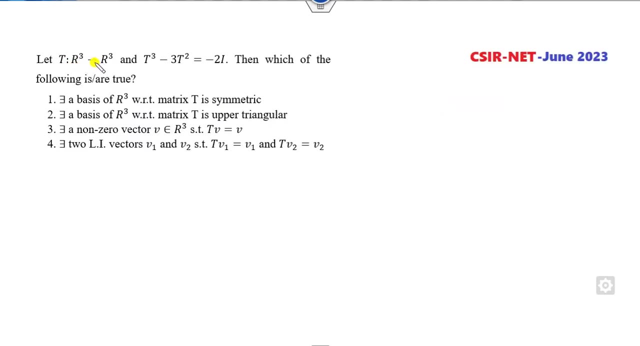 w also has. what is the dimension of the v is my 11, this is my v. dimension of w is also 7, so both have my same. so the right answer is b and d are my correct dimensions. okay, look at this another one. so if t is my r cube to r cube, such that characteristics polynomial is given to you, 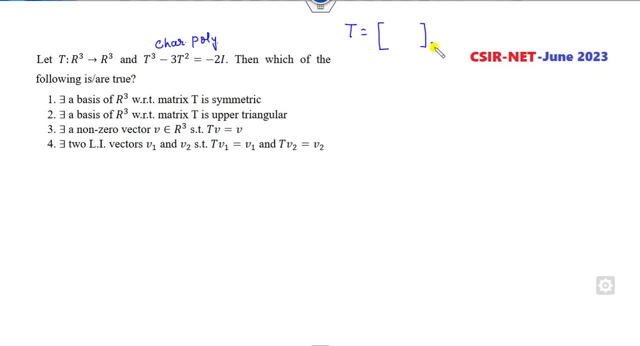 but remember the whatever the matrix, it is not given to you, matrix can be anything which satisfied this property. so if i found the eigenvalues from here, plus of 2 is 0, so clearly says that 1 is the satisfied. so if i apply the horner method, minus 3, 0, 2, 1 is satisfied. 1, 1, minus of 2, minus 2 and minus 2, 0. 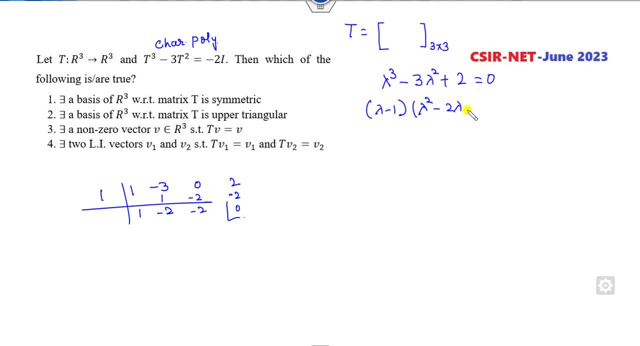 so what other factor is lambda square minus of 2? minus of 2 is 0, then one eigenvalue is 1 second is 2 plus minus 4 plus 8 over 2, so one eigenvalue is 1 second is it's a 12: 1 plus minus root 3. 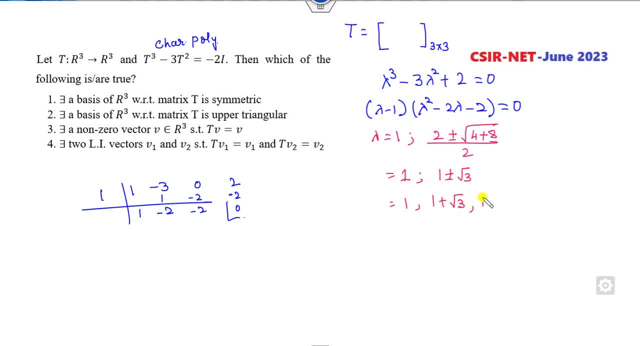 so it means 1: 1 plus root 3, 1 minus root 3. so what is the meaning of that? they are distinct eigenvalues. it means it is my diagonal matrix, so once a is my diagonal, so you can write the eigenvalue as of this nature. fine, so clearly say that, because it is a smithwick. 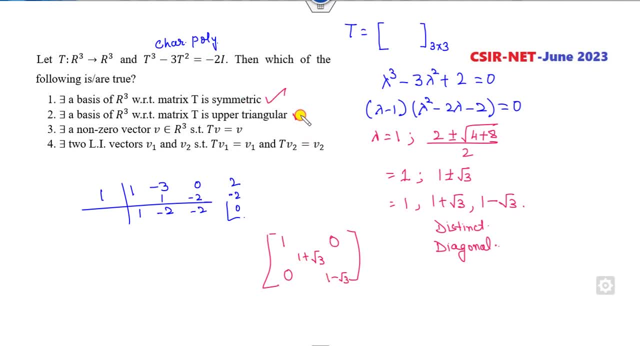 it's the correct option. it is the upper triangular. that's the correct option now, because there exists. so what is the meaning of that? there exists, you can get at least one matrix, so i can simply say: this is my a, whose polynomial is my this one, or you can say t, so one eigenvalue is there one. 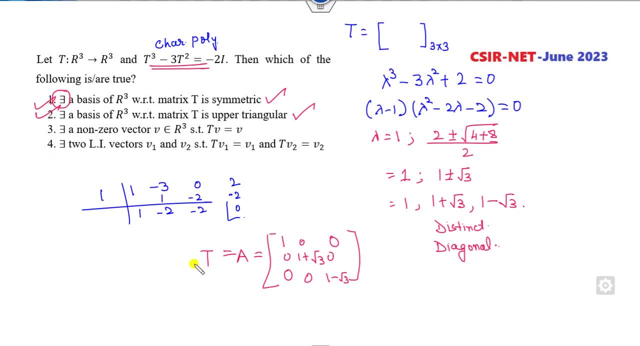 matrix you can found so this satisfied. now, another option is third and fourth. there exists, at least one matrix exists such that tv is equal to v. what is the meaning of that? one is my eigenvalue. you can see that one existence about the eigenvalue. but what is the given original matrix? it is not given to you. 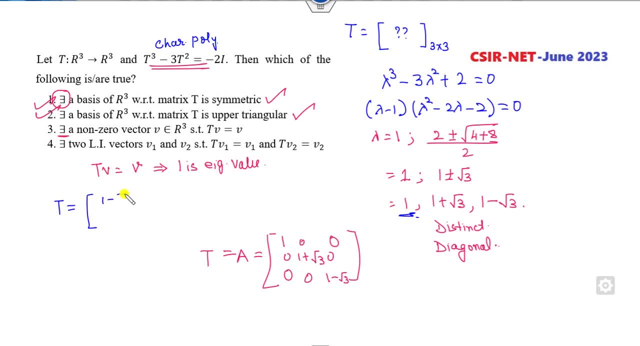 if i simply consider the matrix value as of 1 minus root 3, 1 minus root 3. 1 minus root 3, rest values are my 0. clearly say that it satisfied this, because this is the root of this equation. so this is also satisfied. but clearly say that 1 is not an eigenvalue. 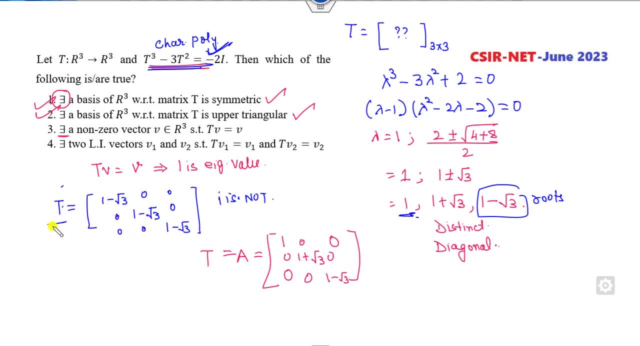 if t is my, because matrix is not given to you. so if you think about this matrix i, i agree you may think about that. if this is matrix, then it is the right answer. but this one counter example is enough to disprove. if i consider this example, 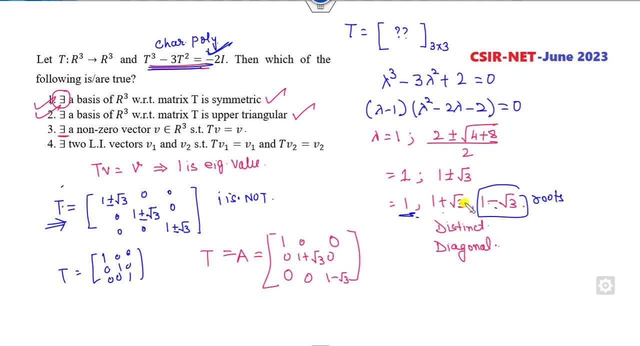 or you can consider any of this case, plus minus of this. both will satisfied here and clearly see one is not the eigenvalue. so this option is cancelled. look at the another case. there exists a Uhr event, a could be my zed by Peter i, or the other way. so it is not the idea. so let me 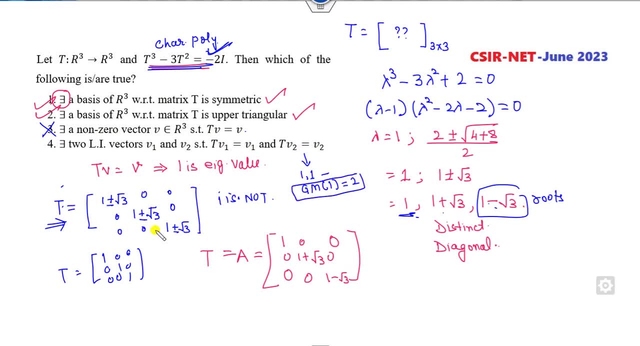 give you some good examples of this one. there is a vector matrix that's the area of the. decorate a random vector value with zed vector k. these are the zed vector's, again the zed vector itself. are the zed vector's screamed by sign of the name zed vector's. so from the zed vector الم. 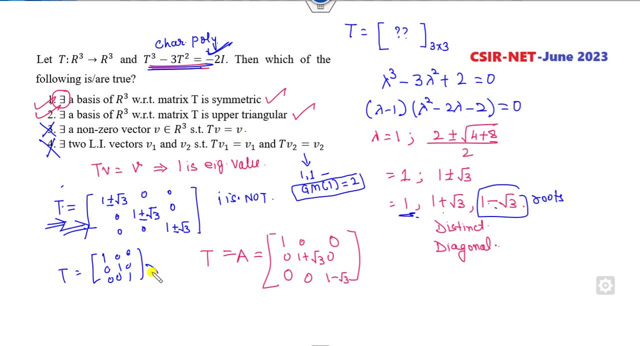 that would be the exact same thing, but that is different thing. from here you can assume the zed vector suite for general input, the zed vector alors certainly say around losin zed vector of 1, or zed vector consortium also with giver mental vector such that p. 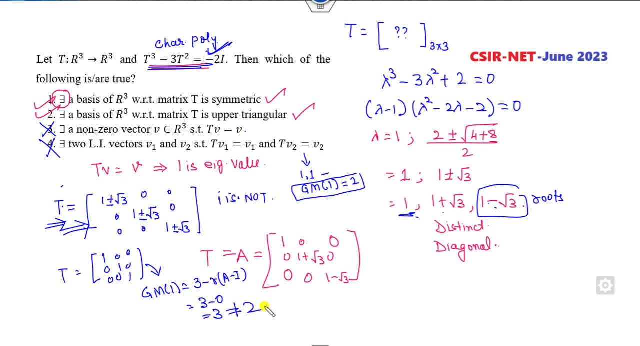 3 minus 0 is my 3, which is not equal to 2. so again, this option is cancelled out. so remember that there is a word of the there exists. so if you consider any of the matrix which satisfy this property, then the third and fourth options are cancelled. so i hope you can simply learn the.